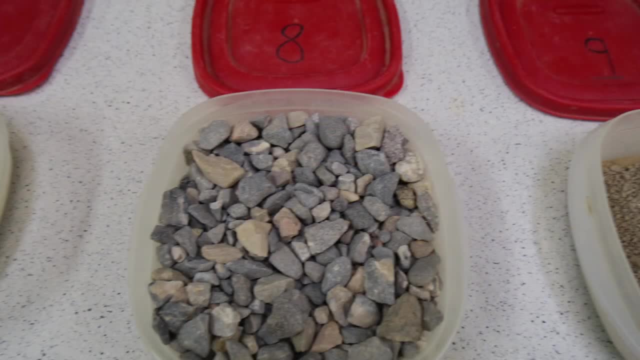 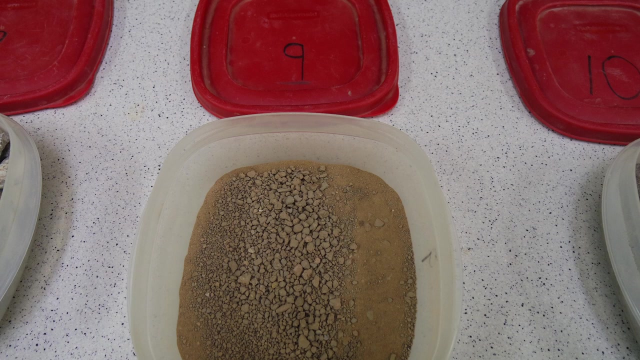 For this lab. I will attempt to describe the soil that you can hopefully make an informed decision on how it should be classified. Refer to the unified soil classification chart in your manual to help you figure out what the material is. Write down your best guess and at the end of this video, 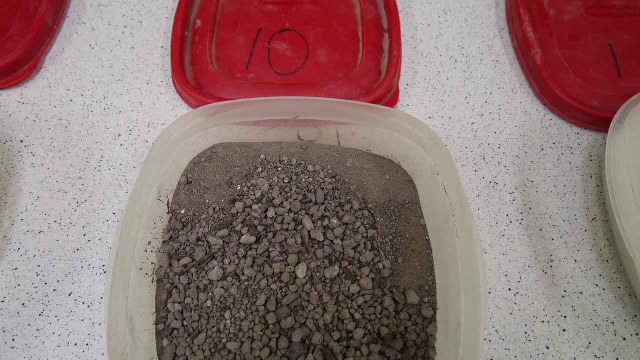 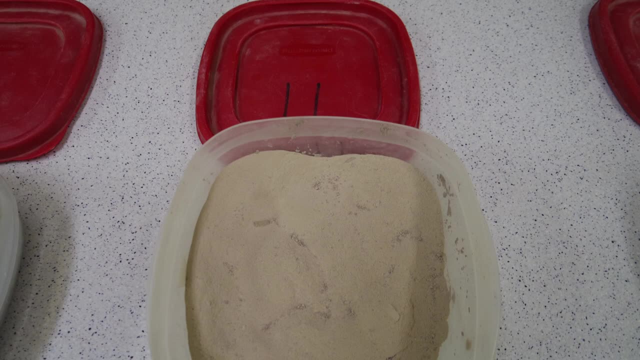 I will go through the samples and classify each of them and tell you why I classified it as I did. There are 12 samples we will go through. Stop the video after each sample, write down your guess and move on to the next one. 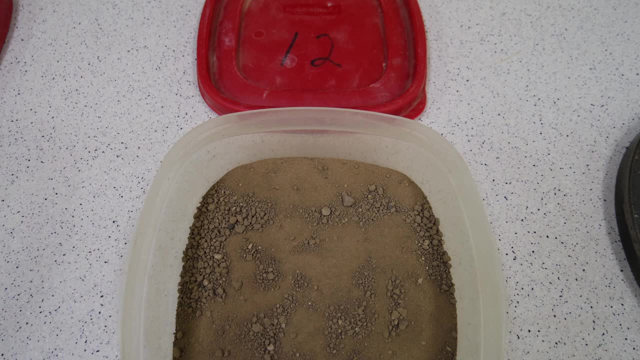 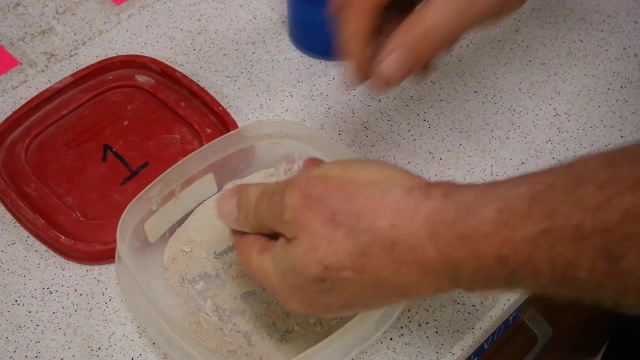 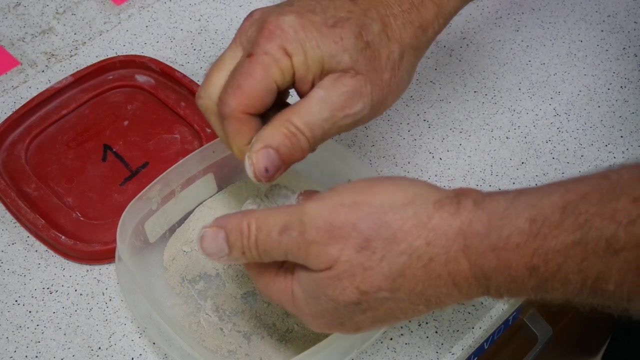 Good luck, and I will meet back with you at the end of this video to talk about them. Okay, this is our sample number one. As I feel the sample, I can feel there are some chunks in it, but they break down pretty easily, and so I just think that they are chunks that are formed from the dried material. 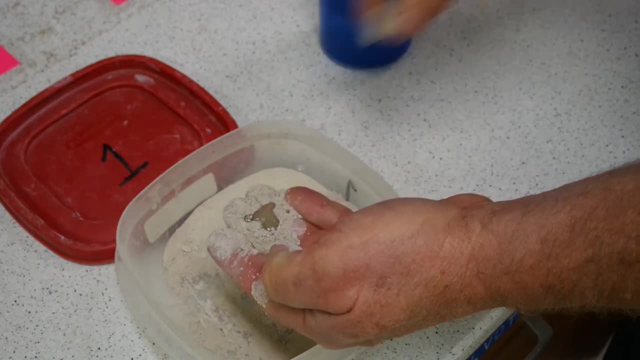 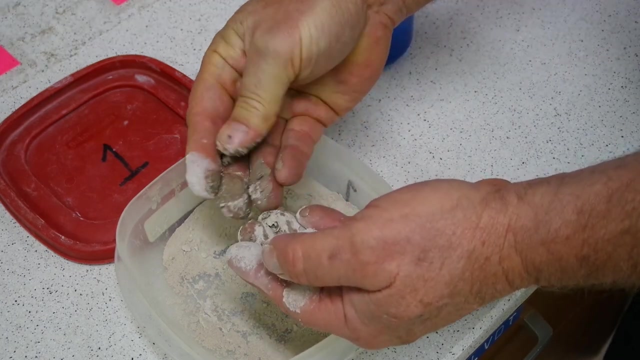 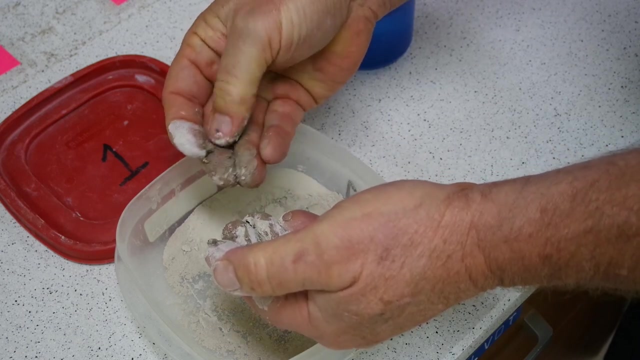 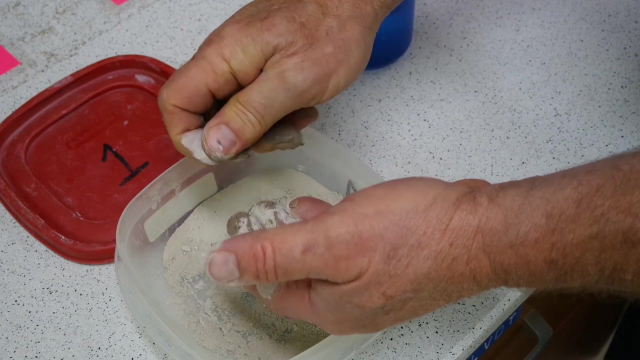 If I add a little water to it, mix it up, I feel that it is fairly silky and because of that, that would tend to lead me to one decision or another on what type of material it is, whether it is a silt or a clay. Looking at this, we know that it is going to be one or the other. 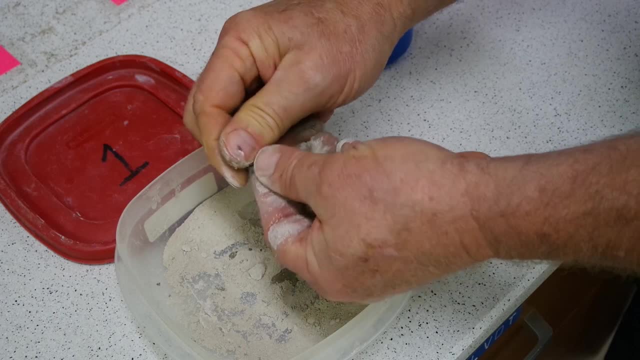 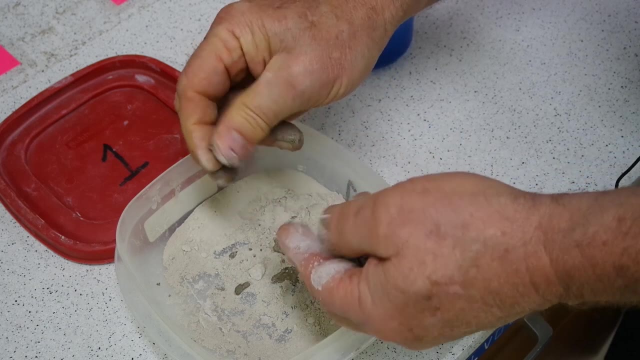 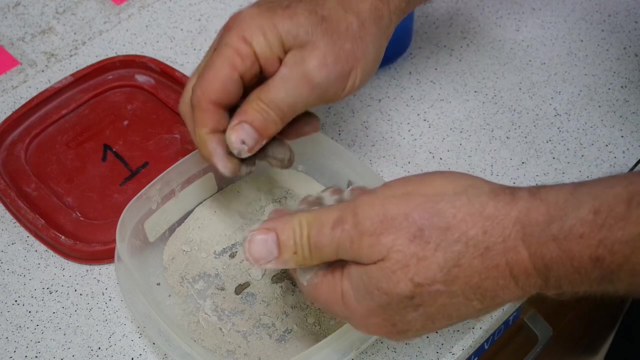 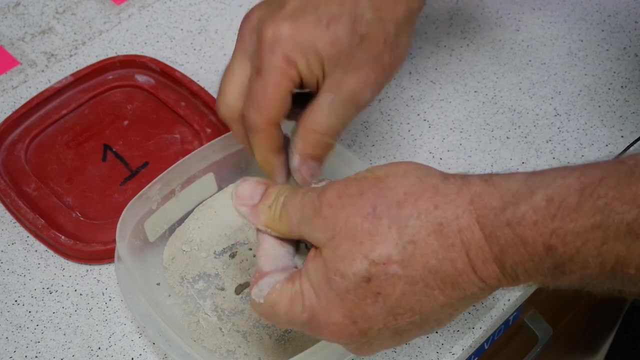 As we roll out the worm, we feel that it takes quite a bit to try to roll it out to where it falls apart. So if that is the case, we know that it will absorb quite a bit of water, And so it feels really silky as opposed to sticky. 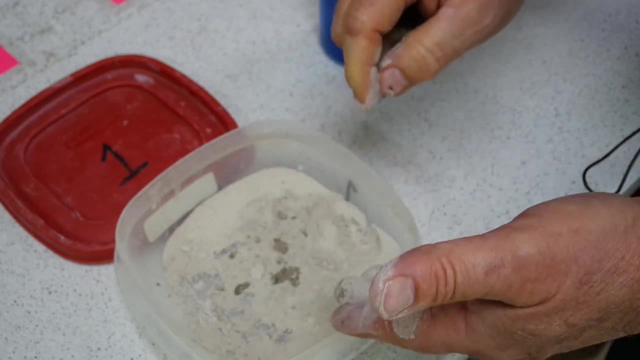 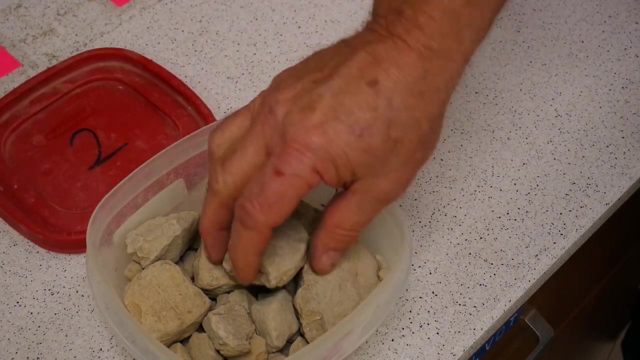 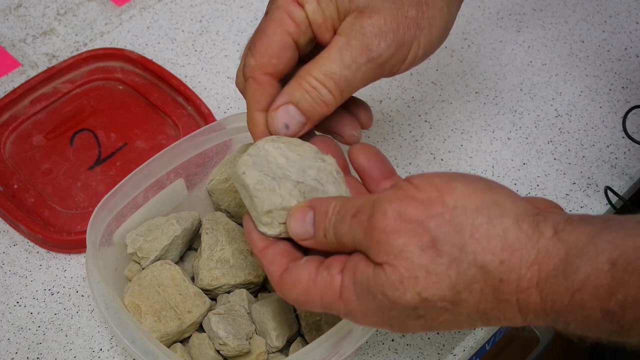 So that is pretty much the description for number one. So this is sample. number two: As you know, it is a very granular material, And so you are going to base your classification on how granular it is. But also we want to look at the makeup of the rocks themselves. 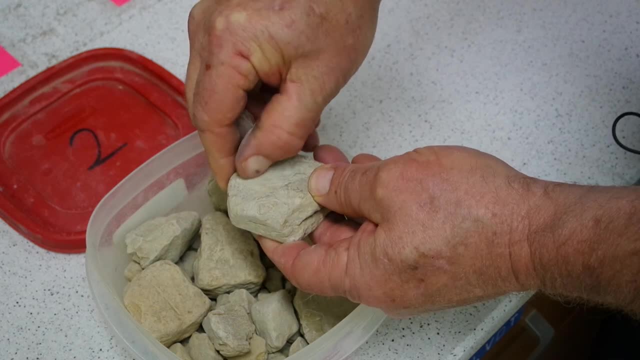 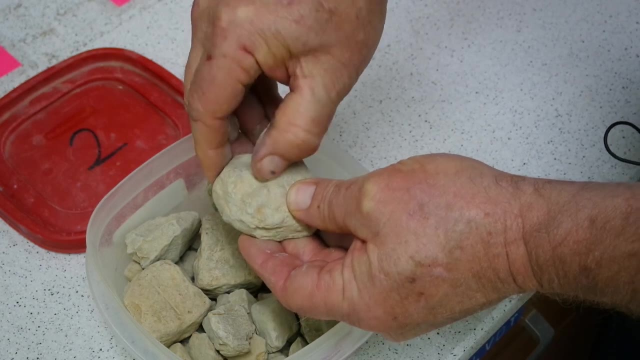 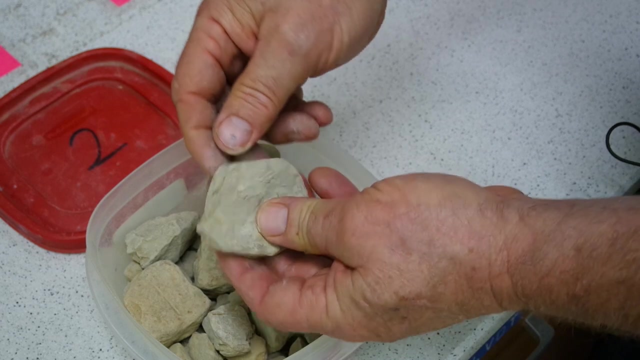 And if you look at this, you probably can't quite see it, but I can scrape the rock off. So, being able to scrape it off, we know that it is not a hard, dense rock, it is something else, And so more than likely, we would be able to break that down. 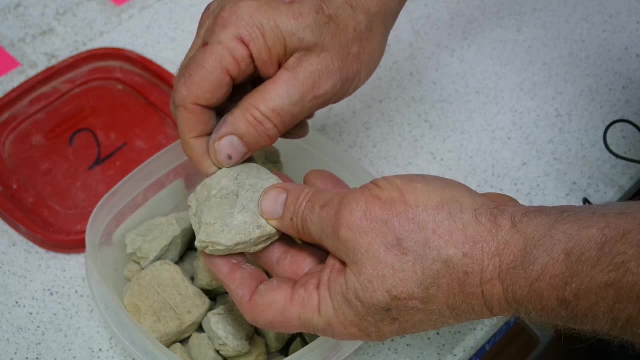 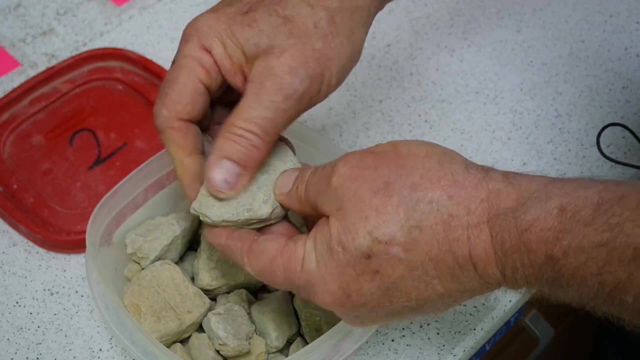 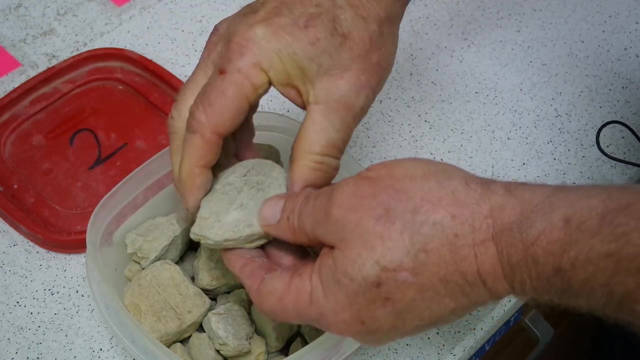 if we had something to hit it with, it would break apart fairly easily. But when it breaks off, it breaks off in really kind of a silky, smooth material And you can see it on my fingers now. Okay, that is number two. Okay, this is sample number three. 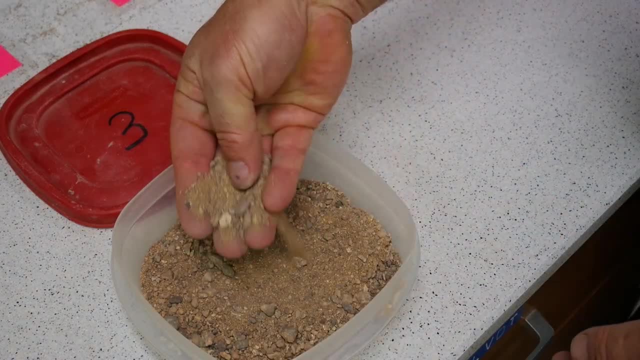 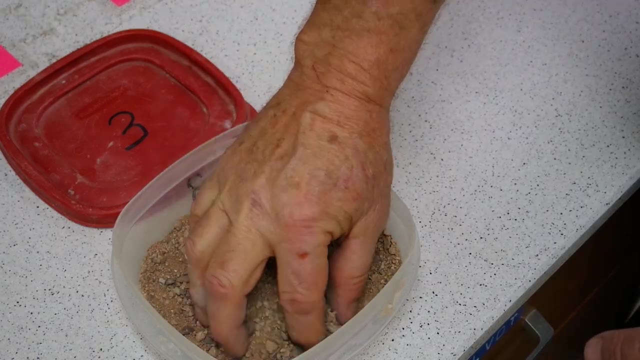 As you can tell, looking at it, that it is a sand. So that is not the question. The question is: how well graded is this sand? Is it a well graded sand? Is it a poorly graded sand? If you look at the distribution of those grain particles? 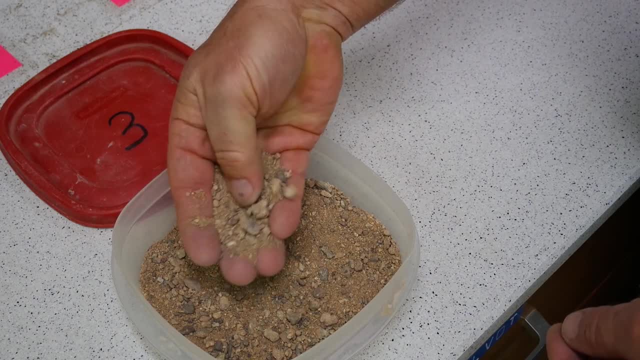 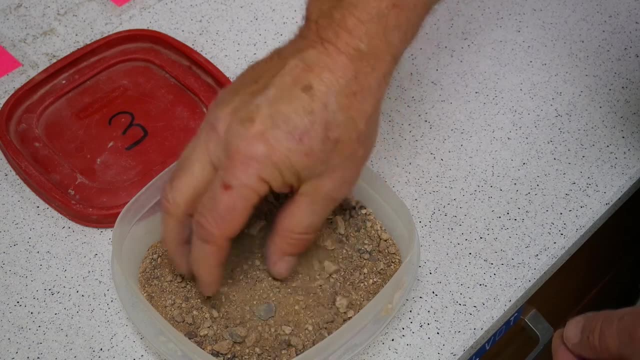 you can get some idea on which way it is, whether it is well graded or poorly graded, And so you have to make a determination on that. The other issue is how many fines are in there. The fines obviously are clays or silts that pass the number 200 sieve. 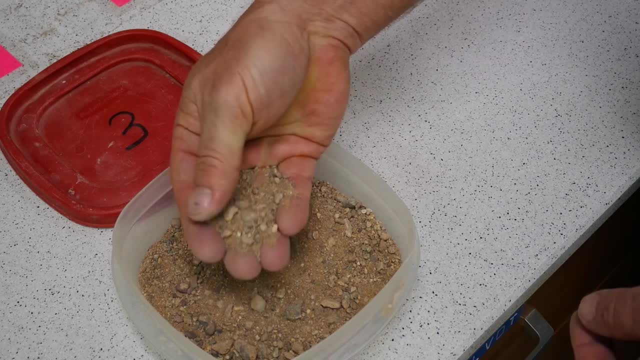 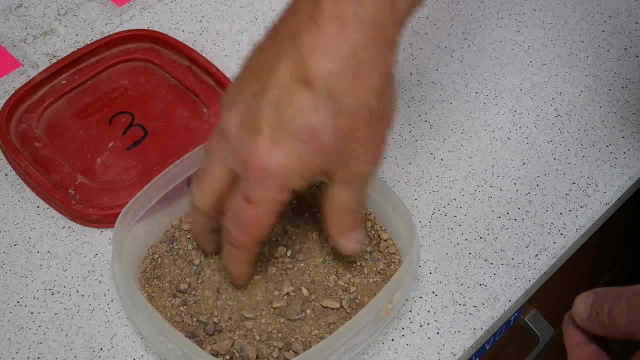 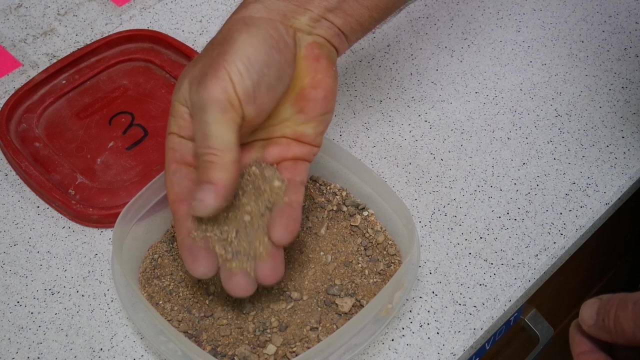 And so we want to know: have we got 0 to 5, 5 to 12 or more than 12% fines in this Which will make a determination on what that material is? If you look at it, it comes apart. you don't see where it sticks together or clumps up. 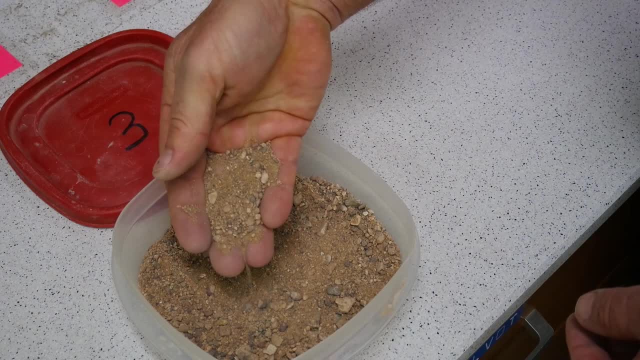 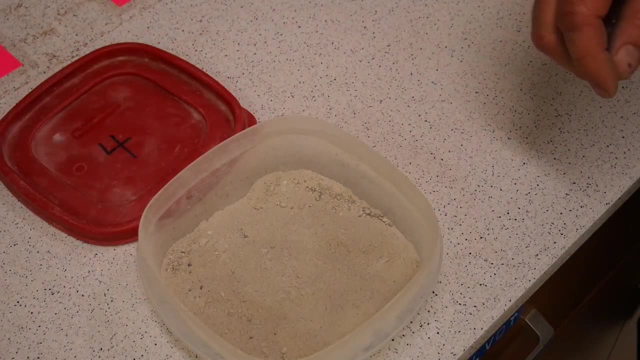 So you know that there is not a lot of fines in there. The question is, how many are there? We will let you determine that one also. Okay, that is sample number three. Okay, we are looking at sample number four. So, as I pull it out in its dry form, 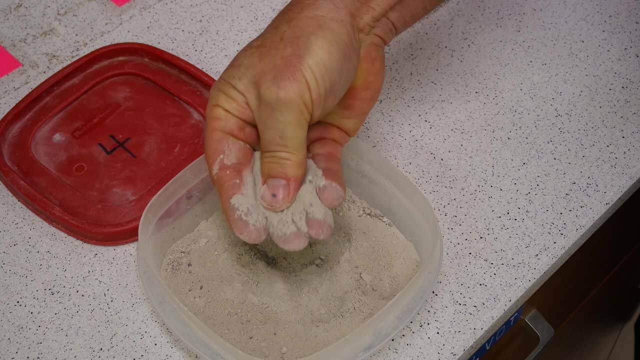 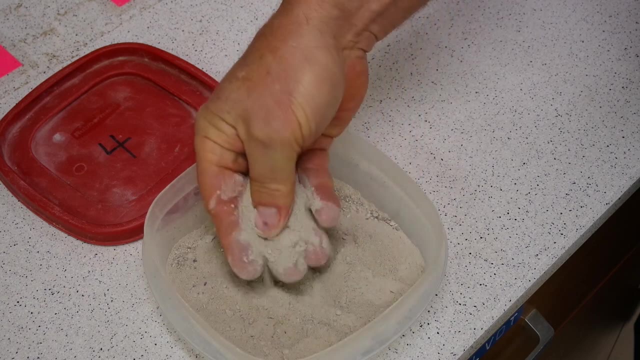 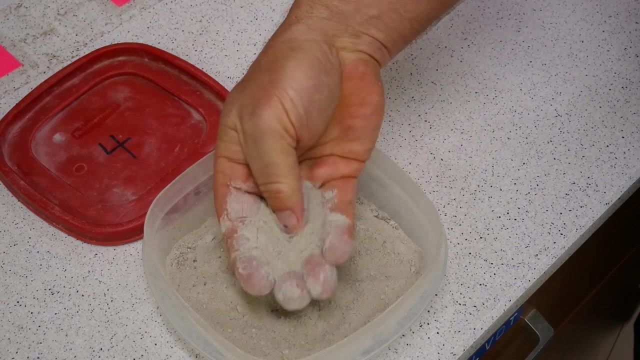 I can feel that there are some sand particles in there, And they are relatively coarse sand. that is in there. I am not sure there is a lot of it though, but there are some. So the question is: is there more than 50% silt or 50% sand? 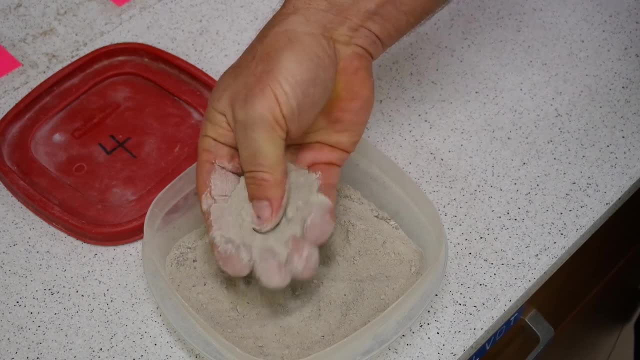 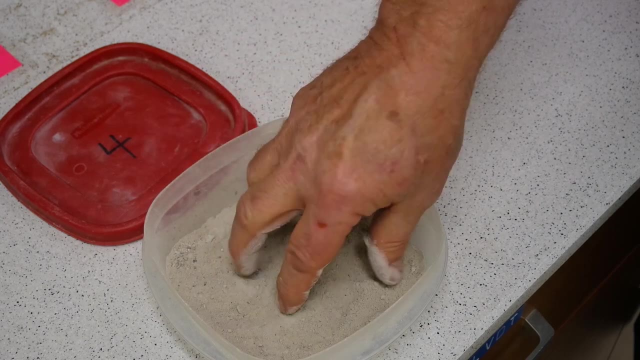 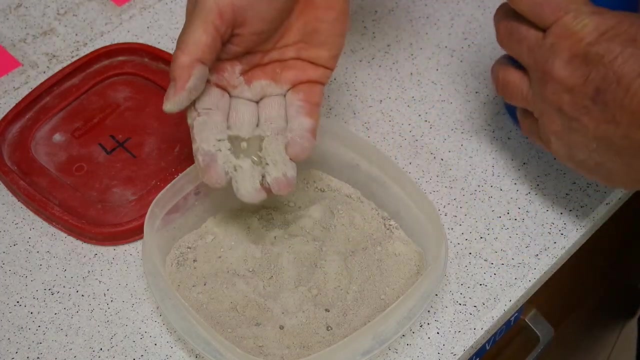 Sorry, not silt but fines, And so that is a good determination on whether it is going to be a clay sample or a sand sample. If I were to look at it because of the material, I would say that you have got a lot of fine grain material in here. 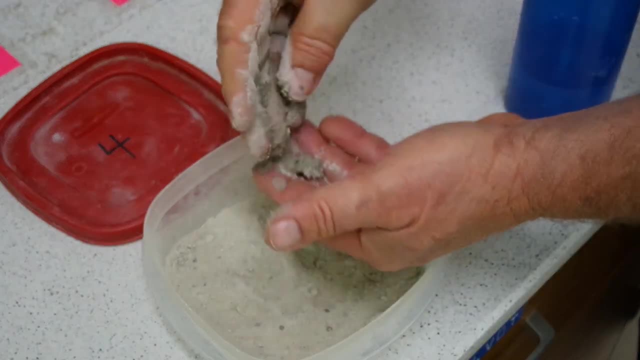 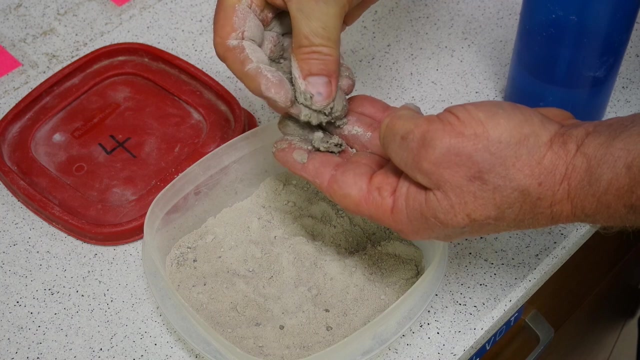 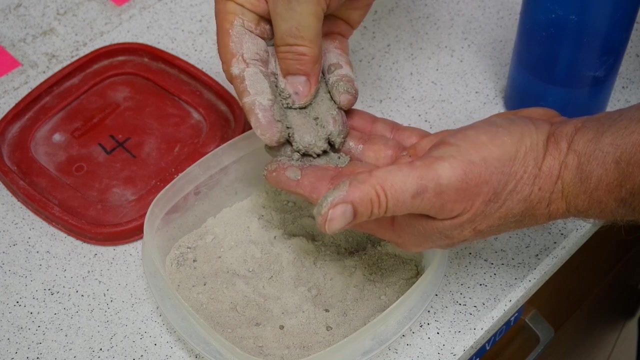 As we put some water onto it and we start playing with it a little bit, we find out that there is a lot of sand in there. You can feel how granular. you can see how granular that material is And feeling it. this is more sticky as opposed to. 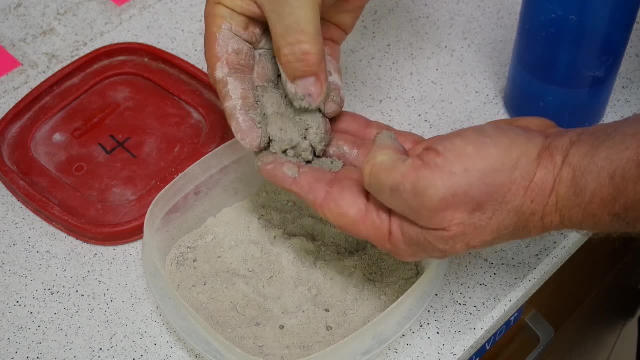 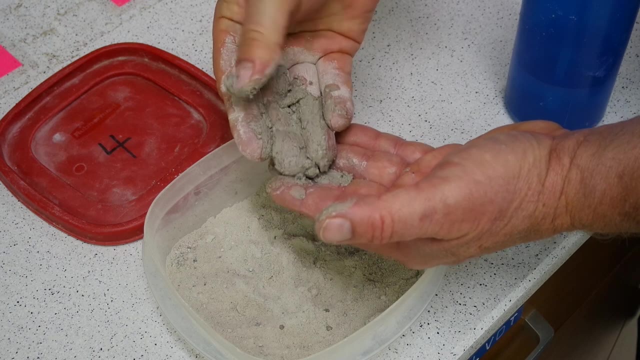 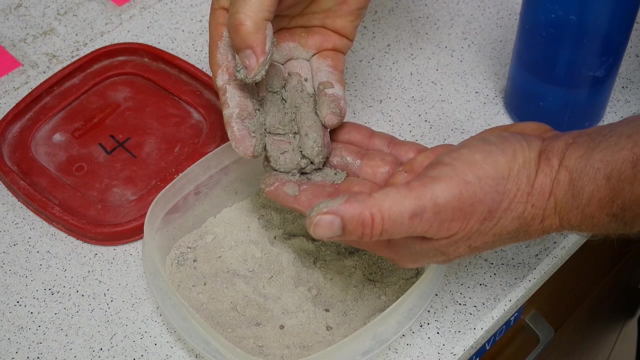 smooth and silky, And so, based on that, you get to make a determination on whether we have got a sand sample, we have got a clay or silt sample, and what the percents of fines are in this. So that is number four. Okay, next we are going to look at 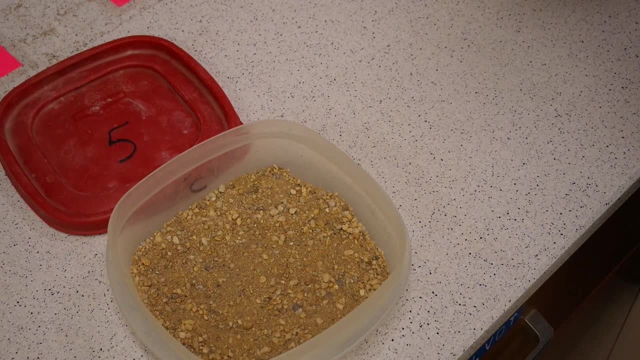 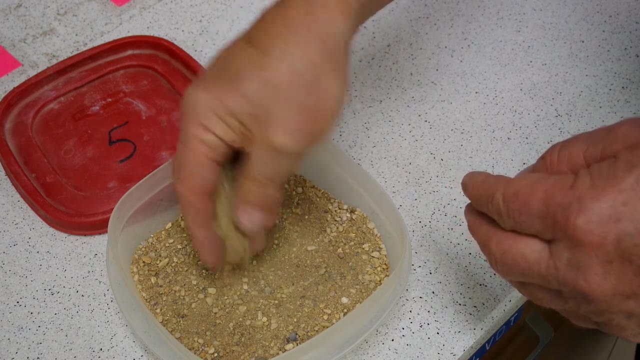 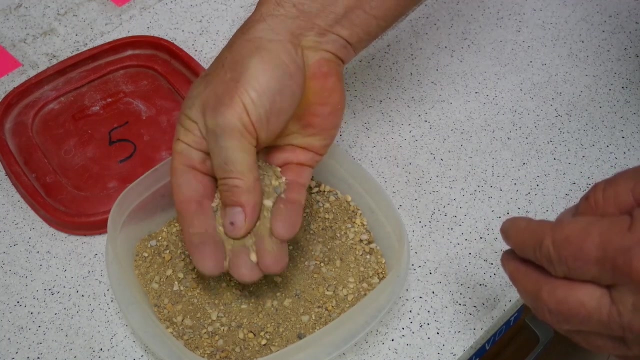 sample number five. As you look at that and if you recall sample number three, this material is very similar to what that material is. Obviously, you can tell from looking at it: it is the sand And, as I feel it, there is definitely some fines in there. 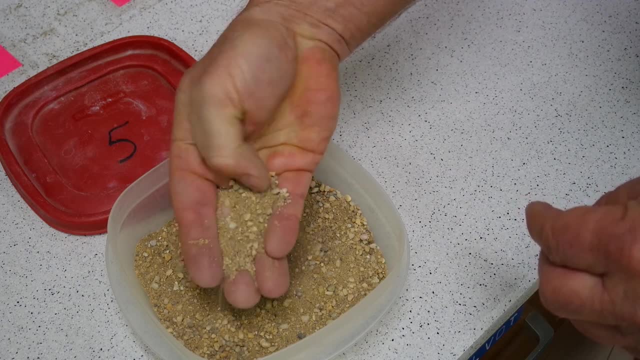 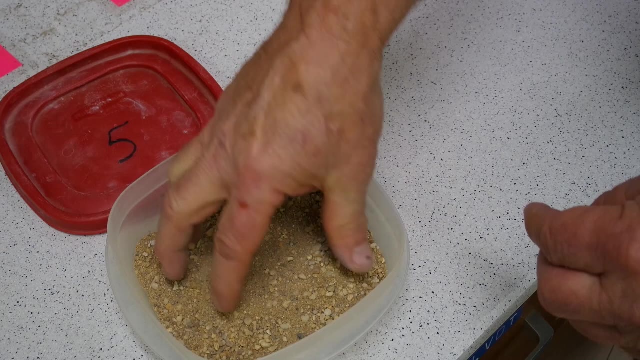 So we have got to decide what the percentage of fines are. If I were to look at this, obviously we know that it is not. there is not a lot of fines, So it is either zero to five or five to twelve, based on your classification. 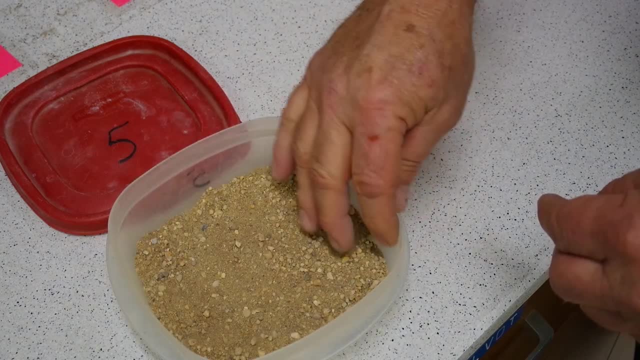 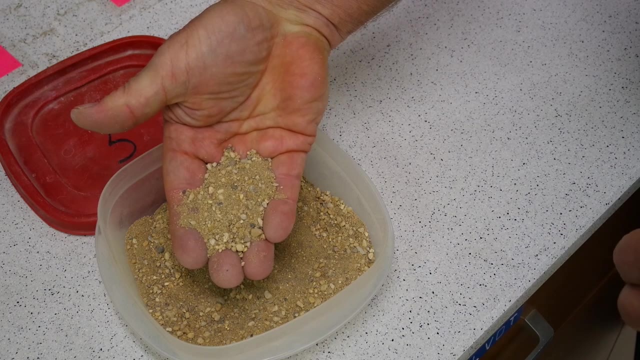 The other issue- we had the same with three: is it a poorly graded or a fine graded sand? So if you look at the sand, you need to look at that and determine: does that look like that is a well distributed material or is it gap graded? 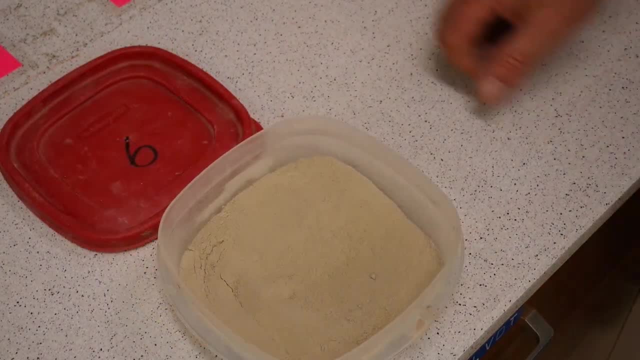 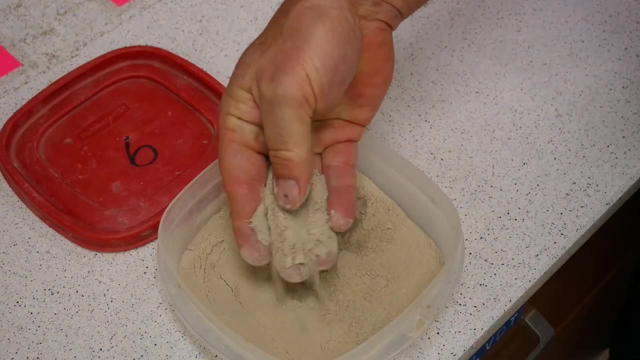 So that is sample number five. Okay, now we are going to look at sample number six. So as we look at sample number six, looking at this, we definitely know that it is a fine grained material. So it is either a silt or a clay. 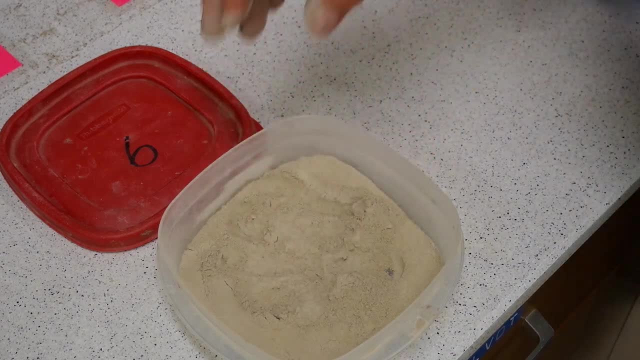 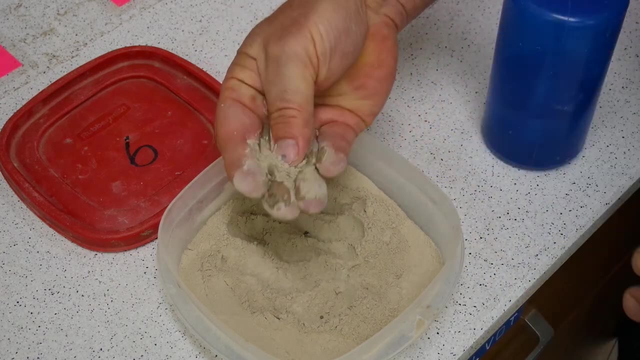 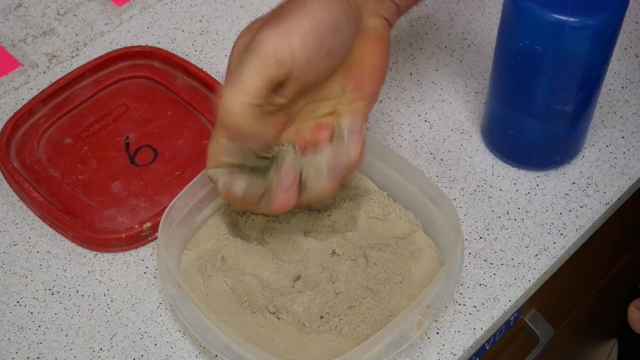 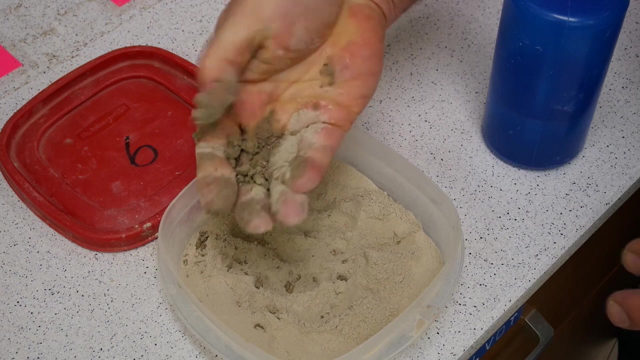 That being the case, we have got to decide which one it is, As I put some water onto it and I start to feel it. I can feel that this sample is really a sticky material And it takes quite a bit of water. I put quite a bit of water on there. 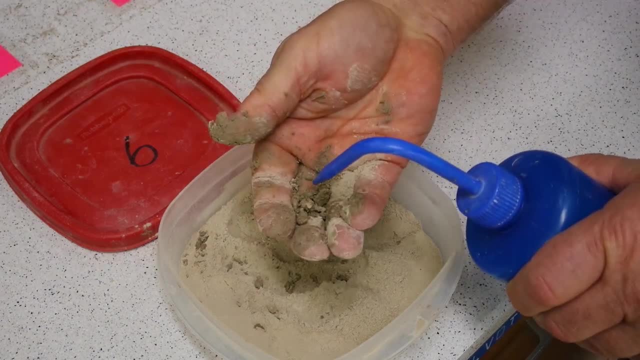 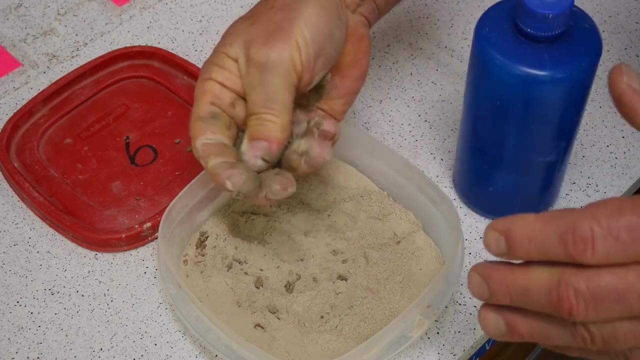 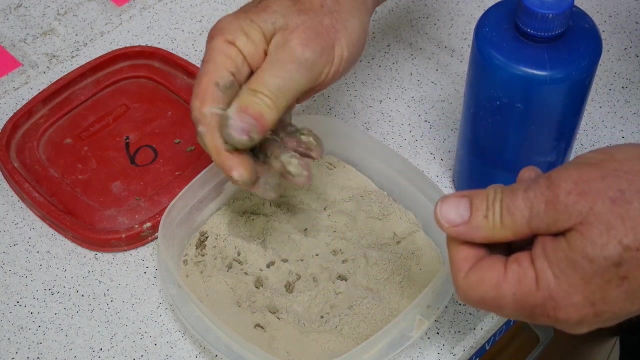 and it still is not quite enough to get it to be into its liquid limit or above its plastic limit state. I add a little bit more water to it and look at this And I start to roll it out. Very easy to roll that down. 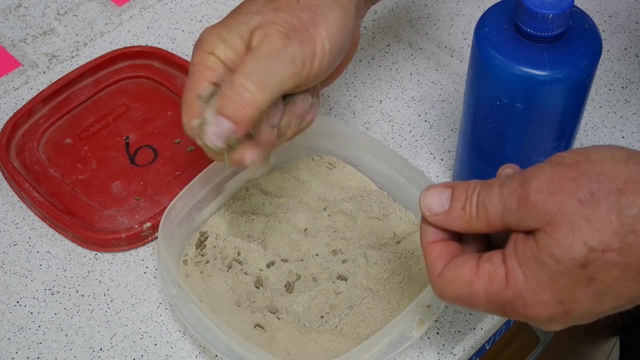 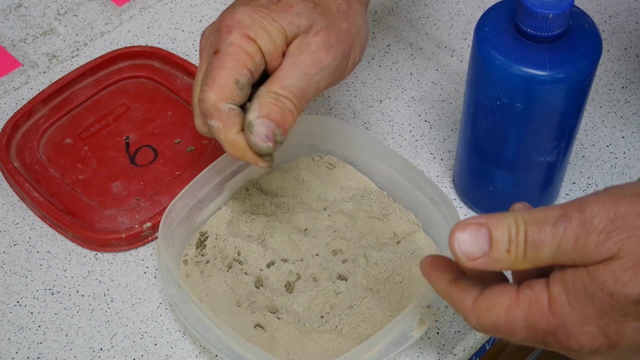 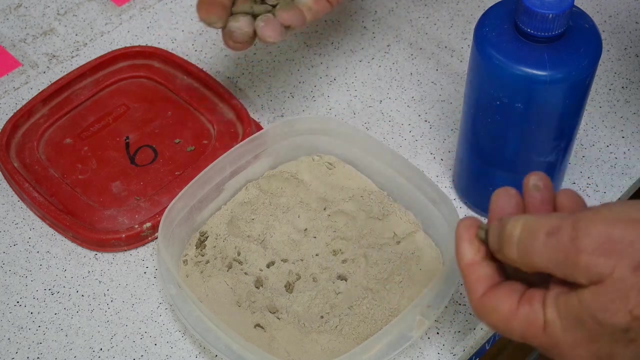 to a very fine little worm here, And so if that is the case- and it took quite a bit of water and it is more of a sticky material than a silty material or a silky material, you can determine what type of material it is. That is number six. 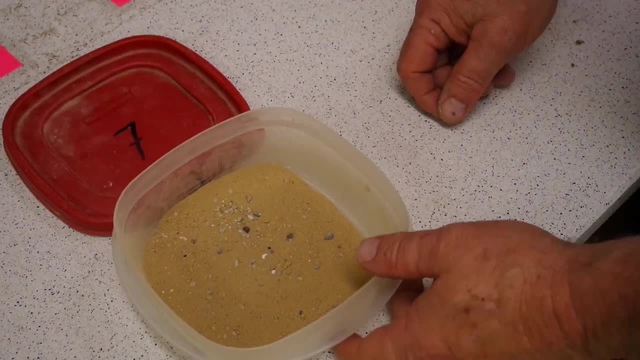 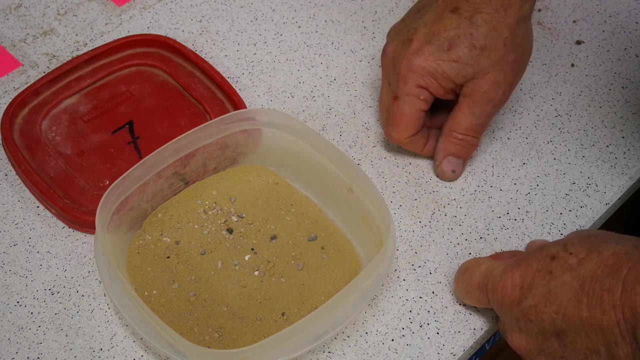 Okay, let us look at sample number seven. So if we look at this right now as a whole, you can see the coarse sand grains that are in there And you can see all of the fines that are also in there. And so, as you look at this, 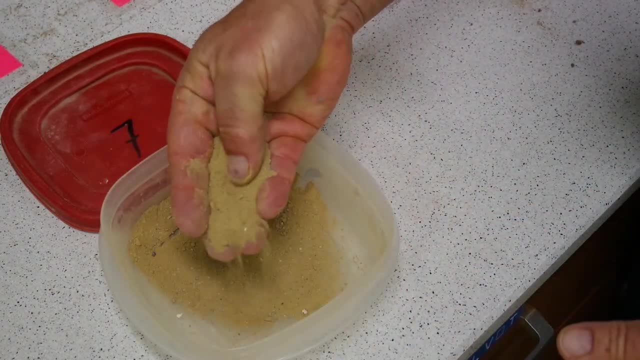 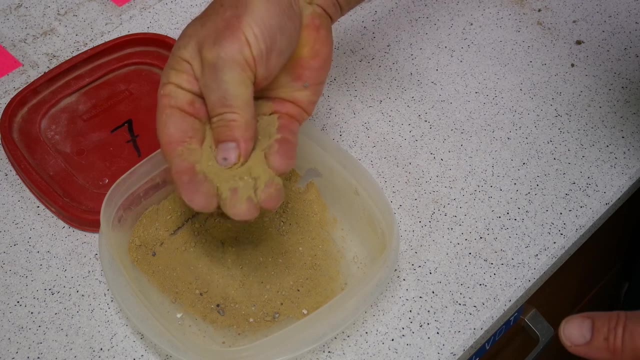 and as we start playing with this a little bit, we need to look at that and say, okay, how much of that is silt, how much of that is sand? And so if you were to look at that, you would say that is probably pretty close to one or the other. 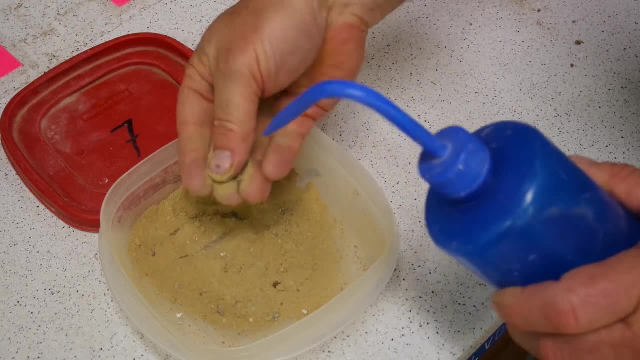 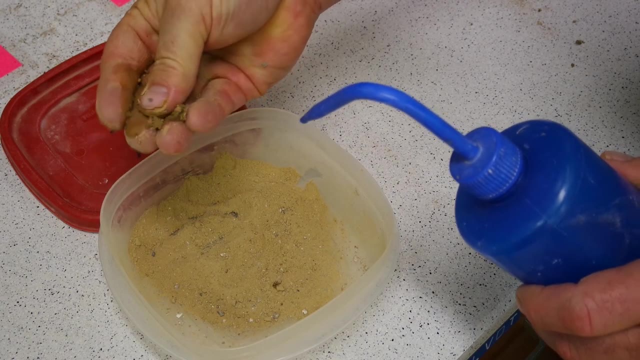 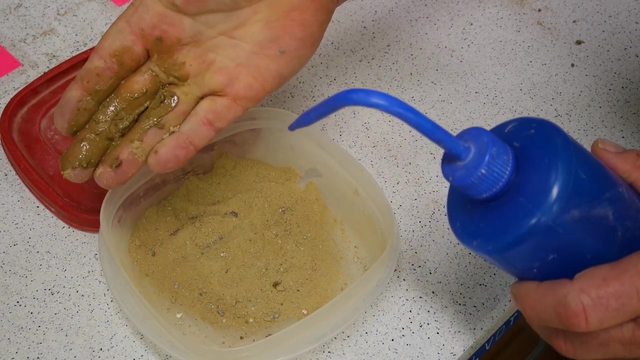 So if we throw a little bit of water on there and we look at that material, we can feel in my hand. I can feel in my hands how granular that material is And there is a lot of sand mixed in there. but if you can see, 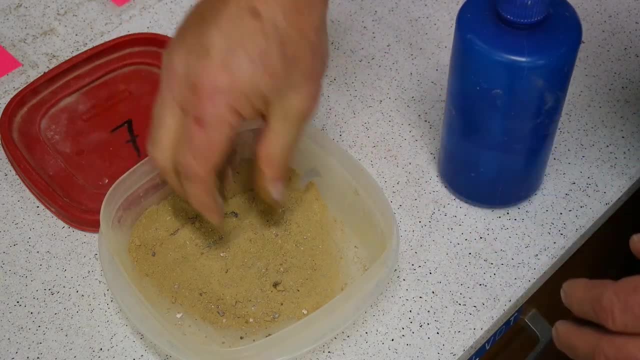 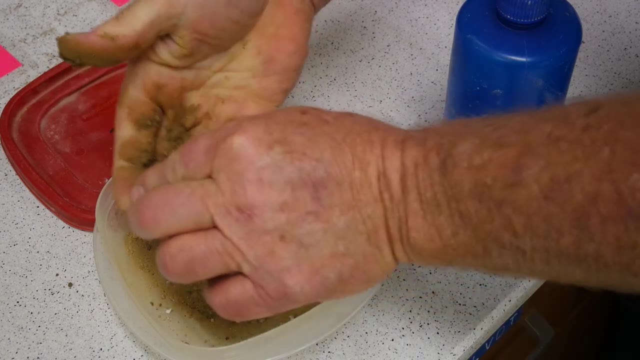 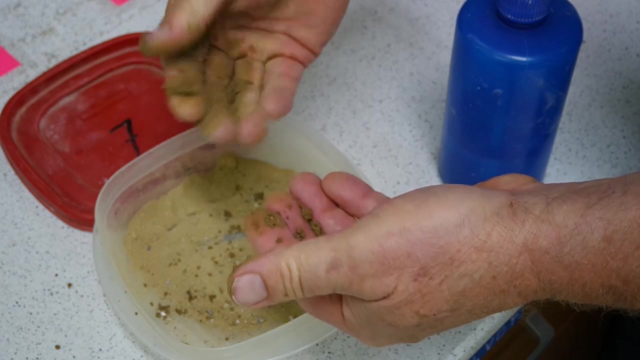 from all the mud. there is also quite a bit of fine material in there, And so if I were to take that and try to roll a worm out of it, I think I would have a hard time getting a worm rolled. In fact, there is no way I would be able to roll a worm out of this. 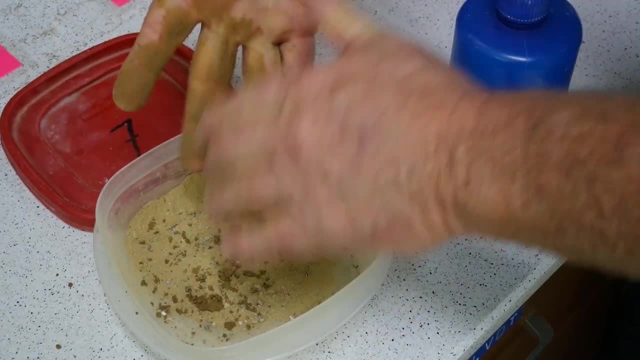 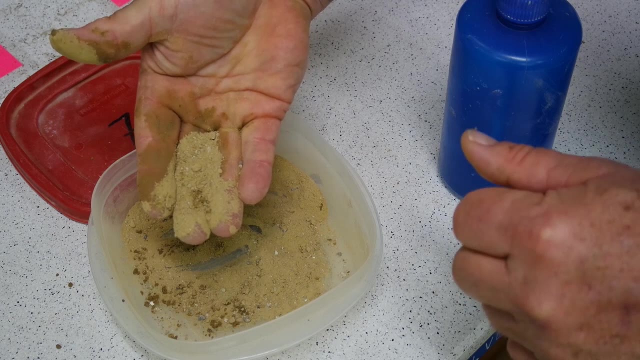 And so it is going to be a non-plastic material, And so the decision that you have to make, based on what this looks like, is whether it has more sand or more silts in it, And so that is going to be your determination. 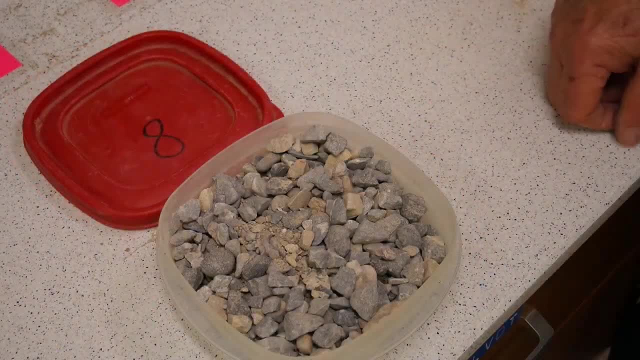 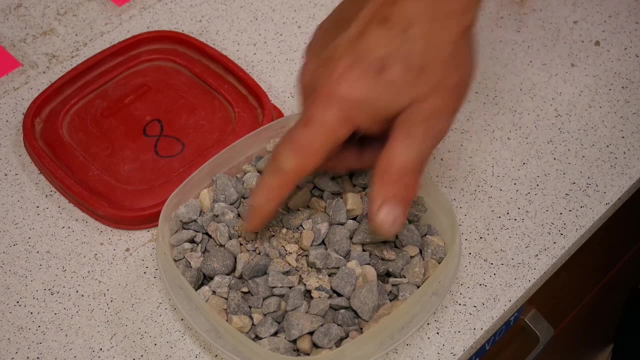 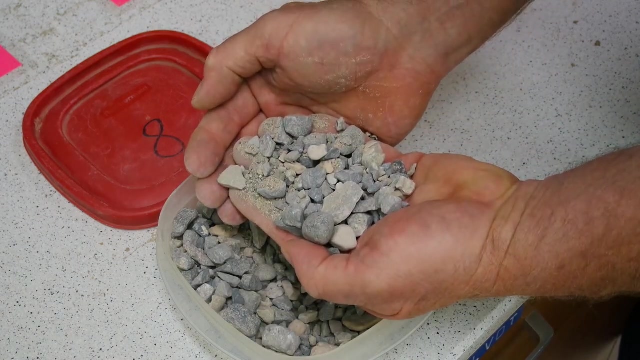 That is sample number seven. Okay, let's look at sample number eight. So if you look at the surface of this, you can tell that it is fairly coarse. If you dig down into it, you can see the fines that are down underneath. that also. 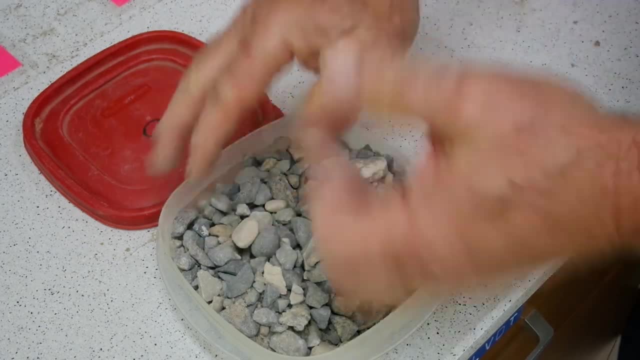 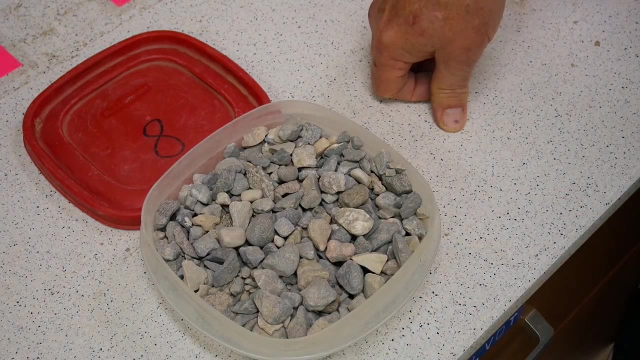 So if you took the sample as a whole, you would notice all of those fines that are down there And so. but as you look at it you can tell there is a lot of coarse material, And so, as you know that the difference between sands and gravels 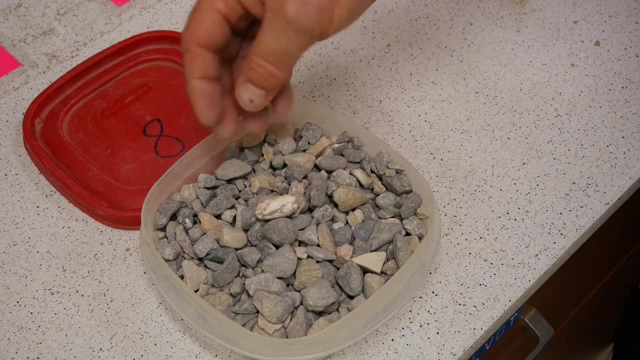 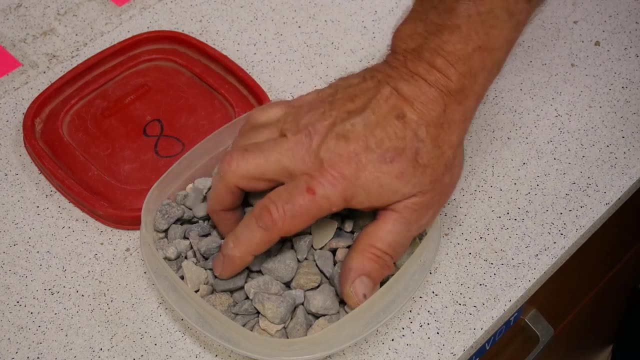 is where it splits on the number four screen. So the decision you have to make is: is there more passing the number four or more retained on the number four? The other decision you need to make is to see how poorly graded or well graded that this material is. 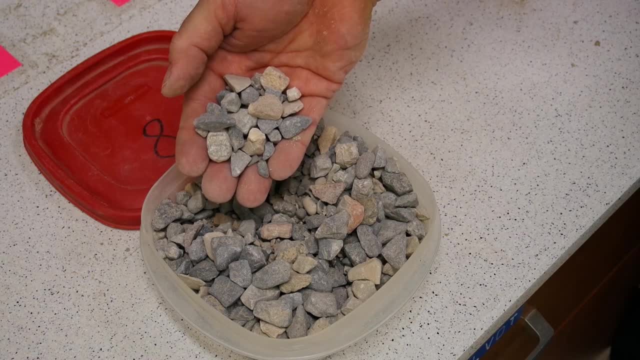 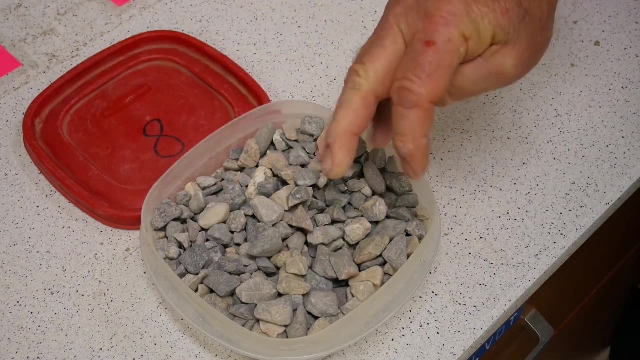 And so, as you look at this, you have to decide whether it is sand or gravel, and if it is well graded or poor graded, So you will be able to hopefully make that determination. That is sample number eight. Okay, let's move on to sample number nine. 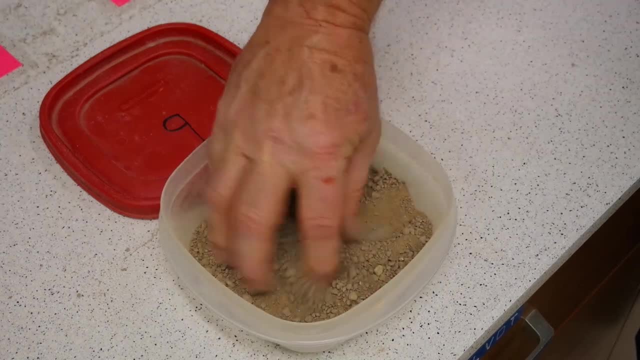 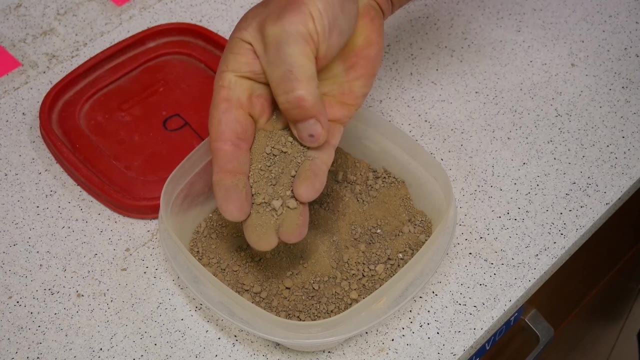 As you look at this, you can see that it has obviously got a lot of sand in it. that makes it a granular material. In fact, as I look at this, I would definitely say there is more sand than silt, as I initially look at it. 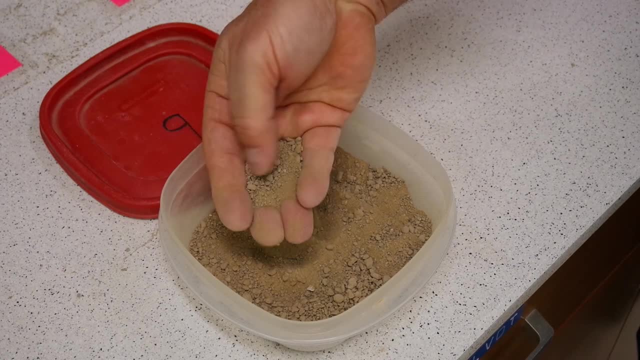 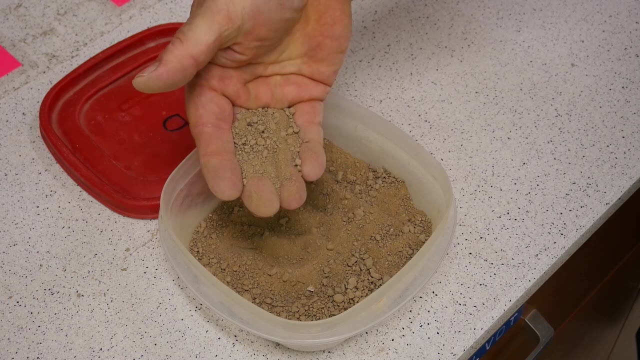 And I keep saying silt, but I mean fine grain, because it may be silt, it may be clay. That is for you to determine. So what you need to determine is is how many fines are actually in this sand sample? So is it an SPSM? 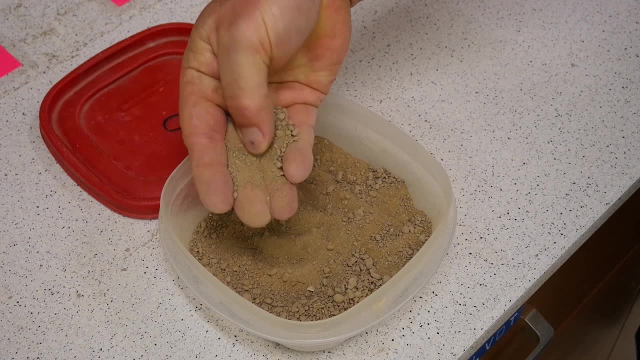 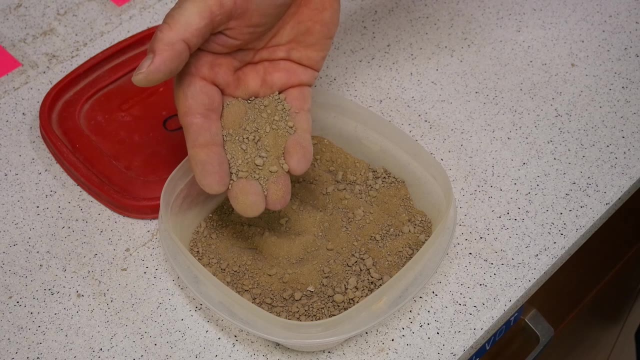 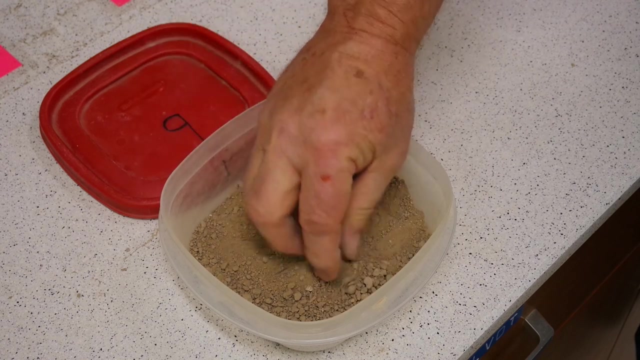 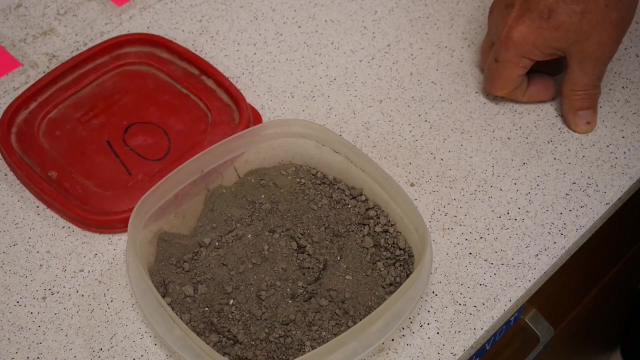 Is it an SM Or is it just an SP? And so, if you can figure that out, obviously, between zero and five, five and twelve and over twelve percent fines is your different classification ranges. Okay, that is sample number nine. Okay, sample number ten. 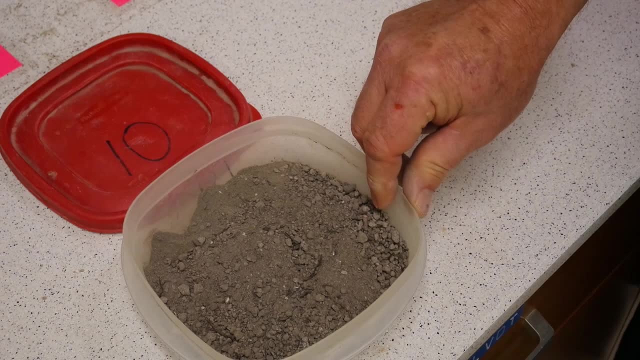 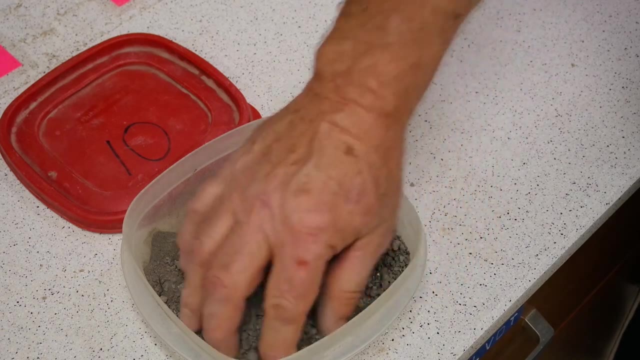 The first thing you notice when you look at this is the different color that it has from the other samples we have had. This is more of a gray material, And so if I were to look at that, I think that there is something in there other than just soil. 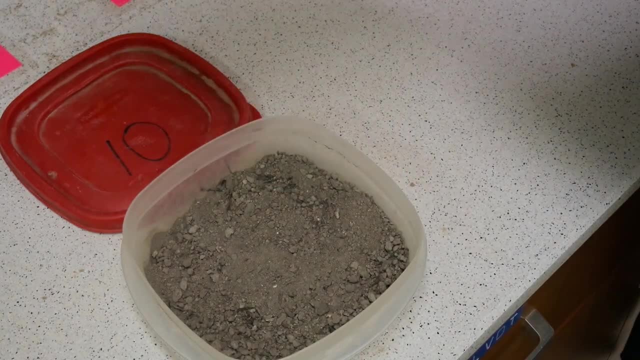 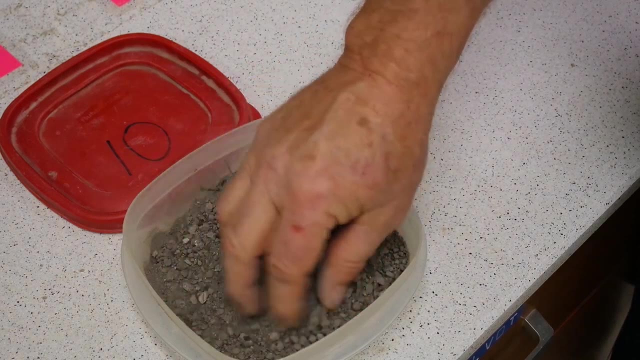 So the first thing I am going to do is go ahead and smell it, And I do get a little bit of that woodsy smell. so there you know that there are some organics in this, And so you have got to take that into consideration. 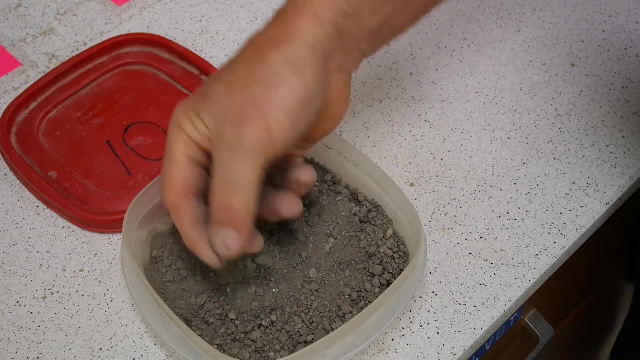 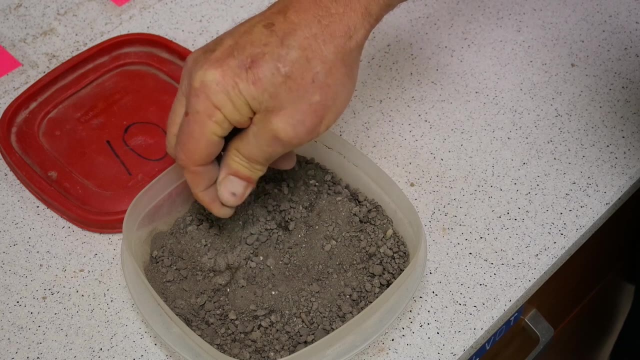 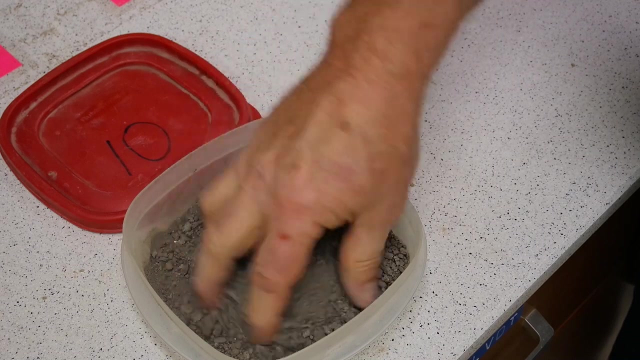 And when you look at these chunks that are in here, are those chunks more organic, Because they break up really easy? Are they more silts or clays, Or is it a, or is it more of a sand material? So, as I am feeling this, 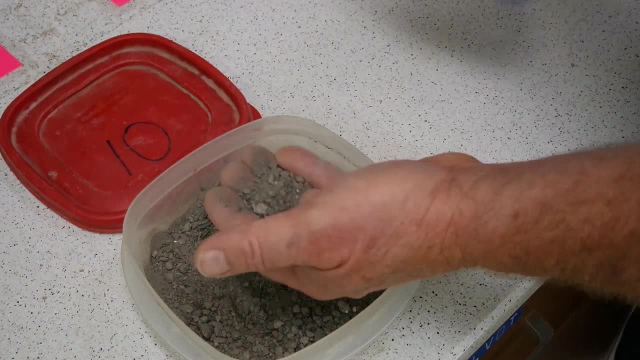 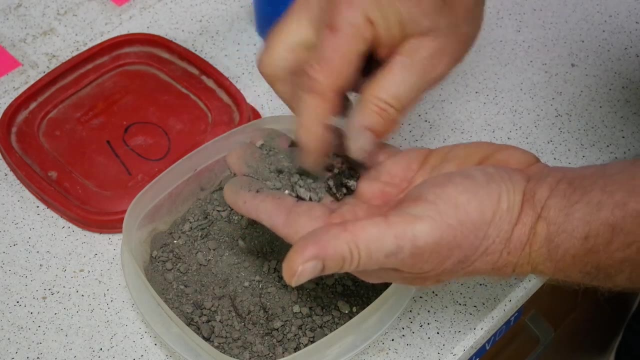 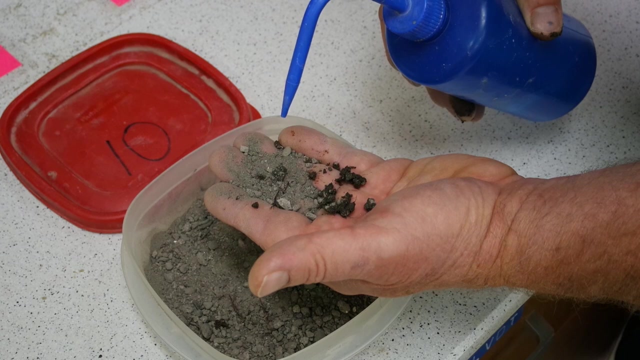 I would tend to think- because it breaks up pretty easily- that it is more of a, more of a silty sandy material as opposed to a, or a silt or clay material as opposed to a sand material. But also, if you look at this, I put water on the top of that. 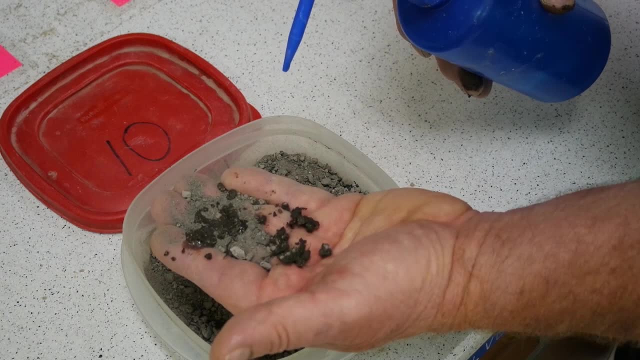 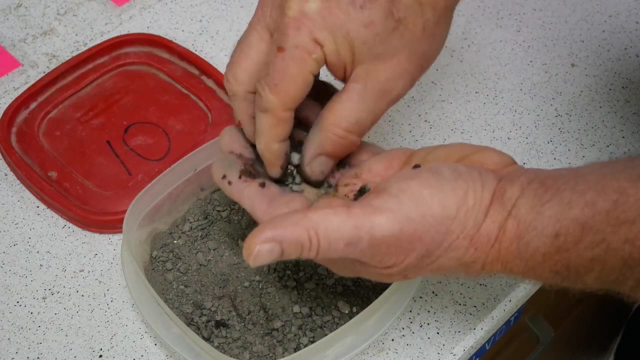 it doesn't absorb right in, it just kind of sits there, Which tells me there is a lot of organics in this material also, And so the determination you are going to have to make is whether it is a. you have definitely got organics in there. 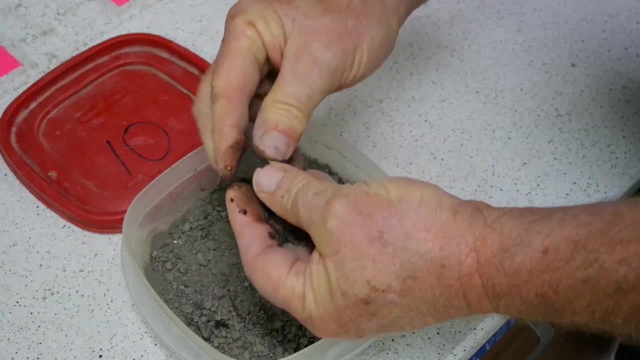 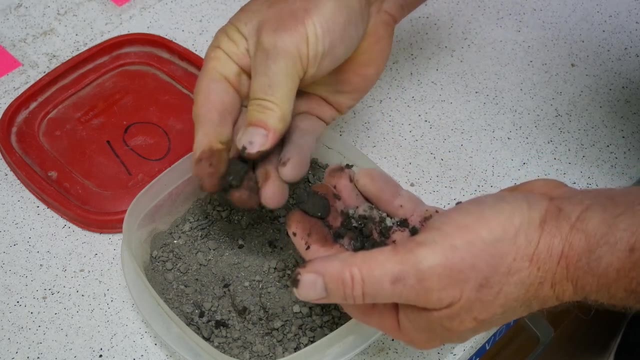 so it has got to be with organics. in fact, as I push this together I can tell I can feel all of the organic material And it broke up and it smashed together pretty well. so there is no more coarse material in what I just played with here. 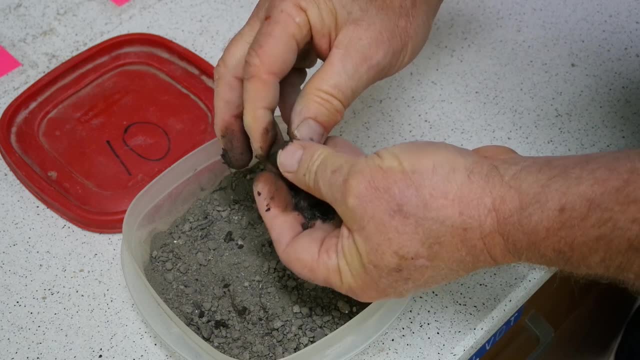 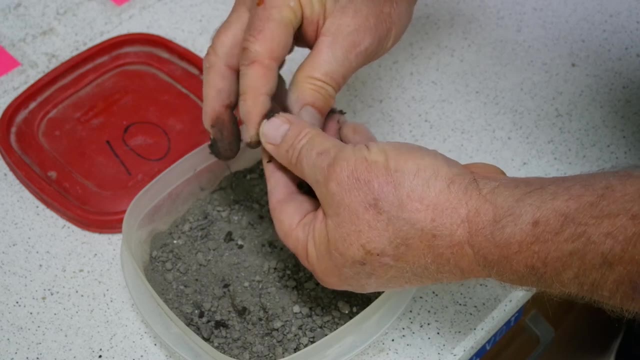 And so really, the determination you need to know is whether it is a silt or whether it is a clay and how much organics are in the material. And we really can't tell what the organics are without our organic loss of ignition or an OLI test. 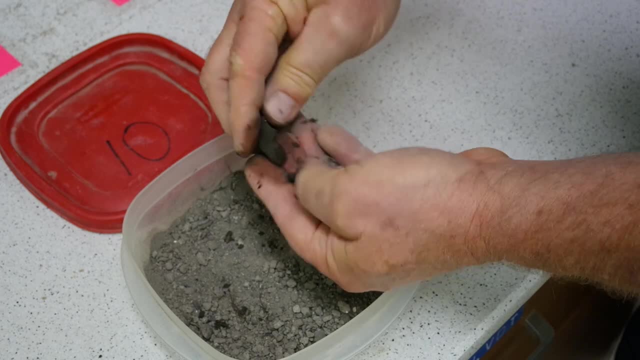 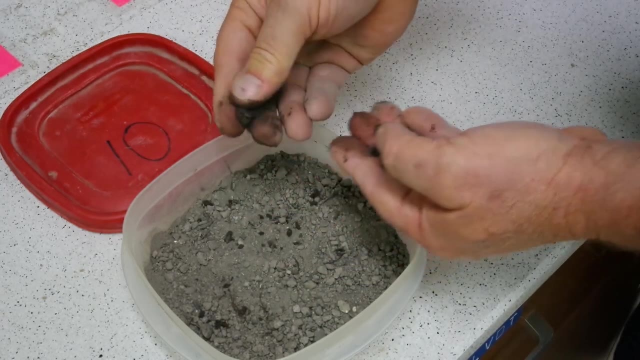 which we burn off the organics, and then we get a weight difference on there. And so, seeing how we are not going to do that, we just have to look at this and see how we want to classify it. Okay, that is number 10.. 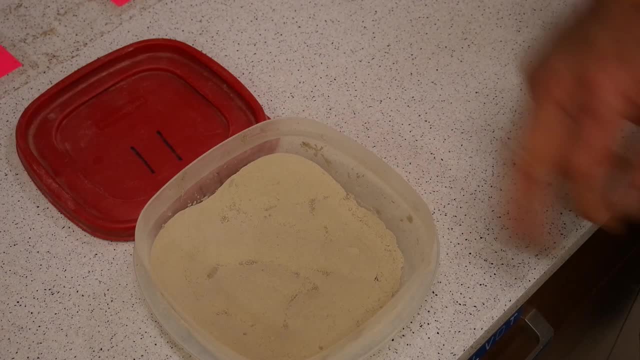 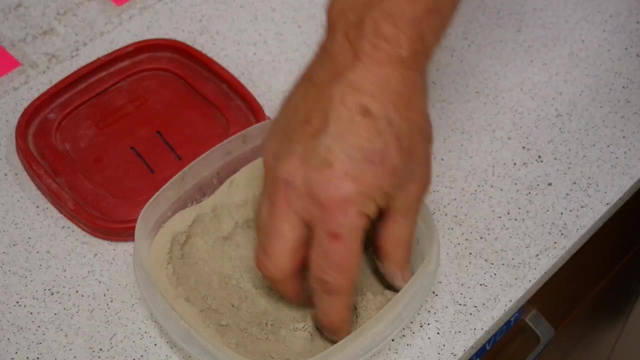 Okay, sample number 11.. So as you look at that, you can tell that it is a fine grained material, And so it is either a silt or it is a clay. So the two things you have got to decide on, first of all, which one of those it is. 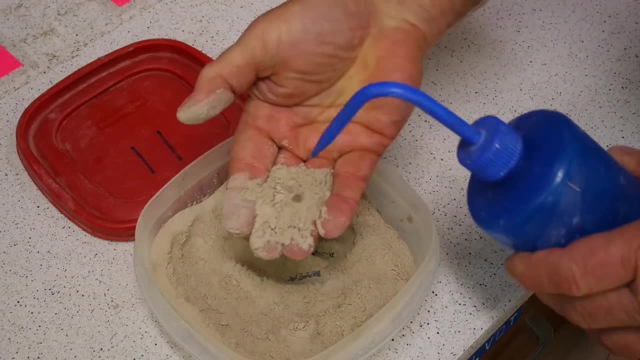 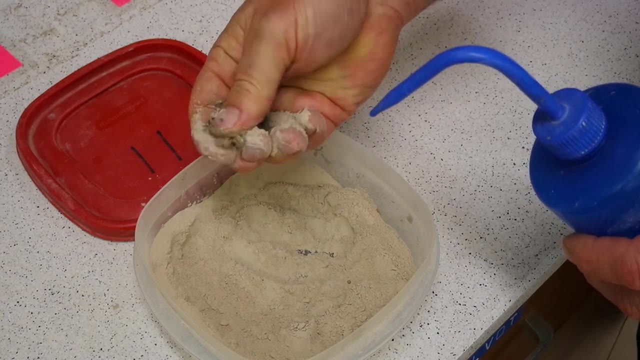 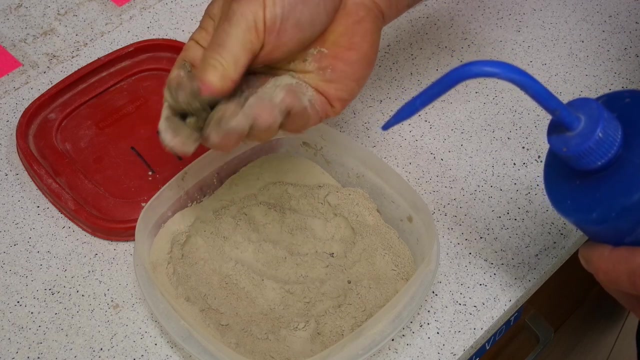 and how plastic the material is. So, as I put a little bit of water onto it and I play with it, it is a pretty sticky material. So, as opposed to being silky, it is pretty sticky, And clays or silts are either one of those. 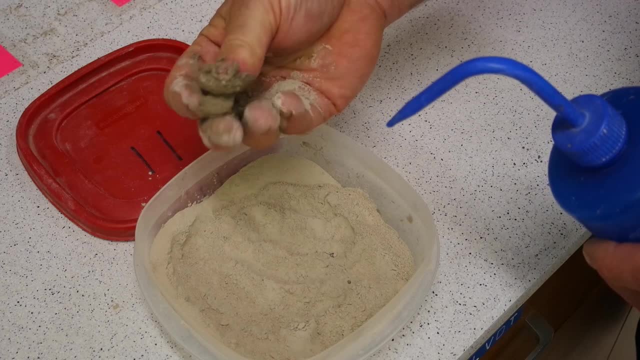 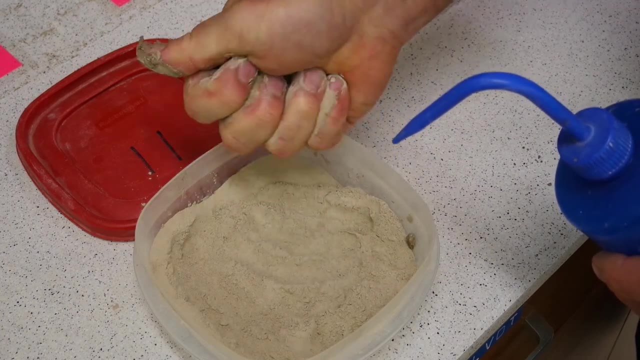 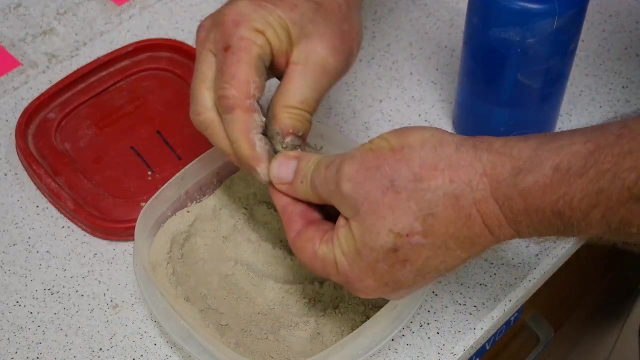 either silky or sticky, So you can figure out which one is which. Also- and I did it- I put a lot of water in there and it needed more material in there, so it didn't absorb a whole lot of water, But I can roll a worm out with it. 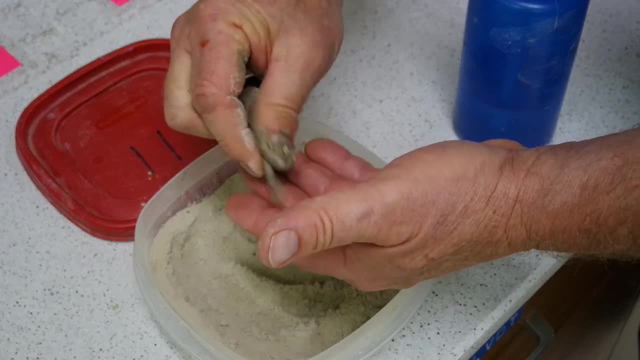 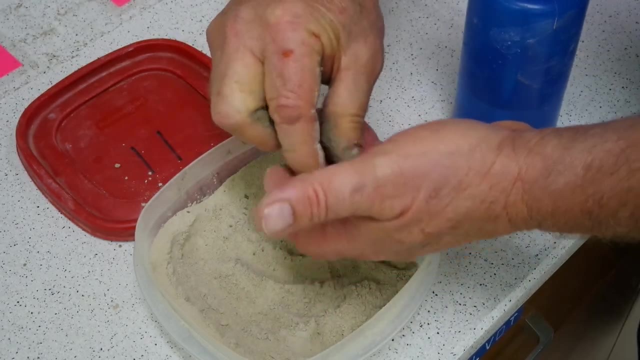 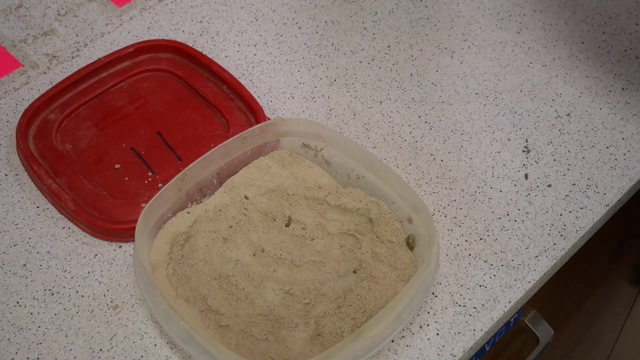 so I know that it is plastic, But not taking a whole lot of water compared to some of the other samples and the fact that it is more sticky than silky, you can determine what this is. Again, that is sample number 11.. Okay, so let's do our last sample, number 12.. 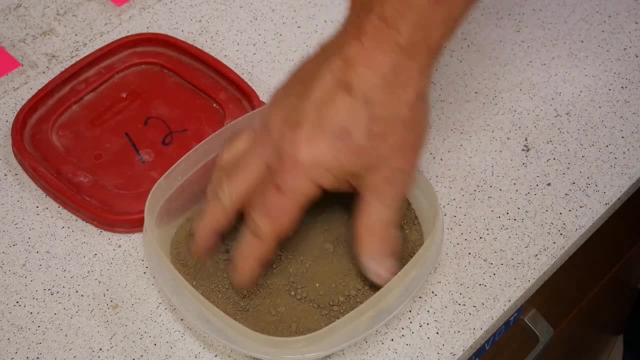 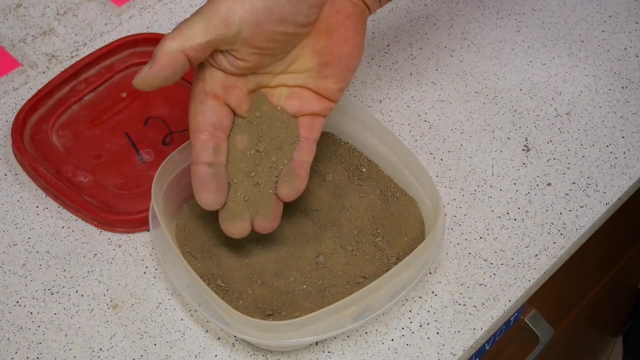 And so, as we look at this, you can see the color. it is a nice brown color, so it is looks like all it is is soil And as you look at it, you have to decide how many fines versus how much sand is in this sample. 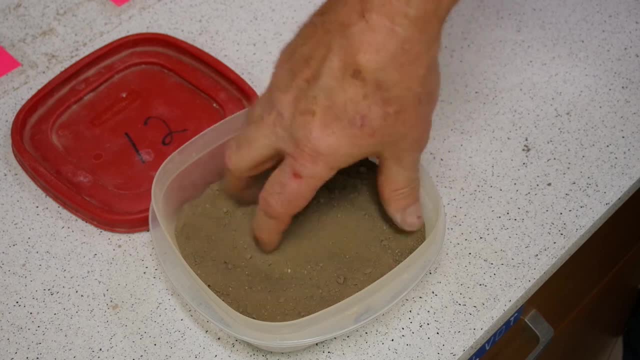 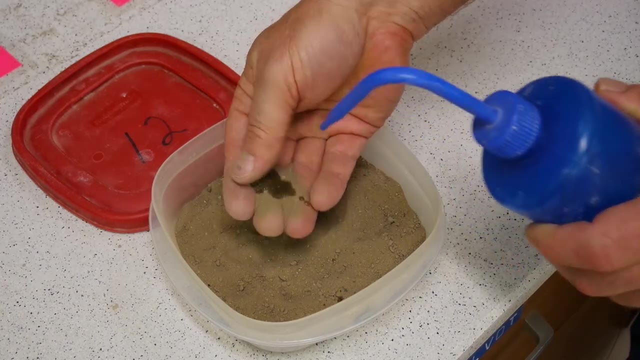 Because we know it has got to be one or the other. It is either a silt clay or a sand sample, And so if I were to put a little water on this, see how readily absorbed in there. and if you look at this, you can see all the grains. 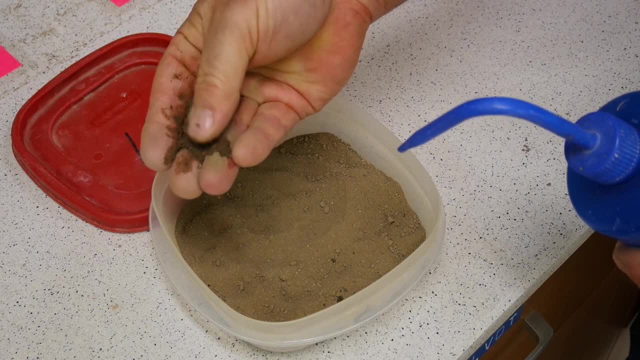 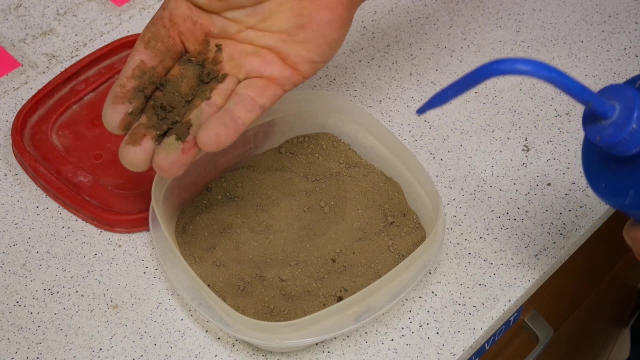 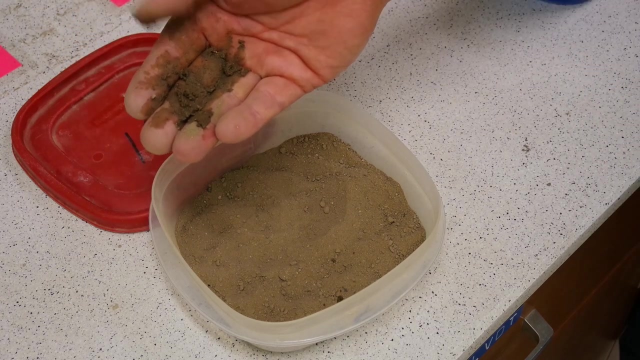 that are in that sample, But there is some binding in there, And so if I were to look at this and feel this, I would say there is probably more sand than there is fine materials in that. So you have got to decide whether it is a sandy clay, a sandy silt. 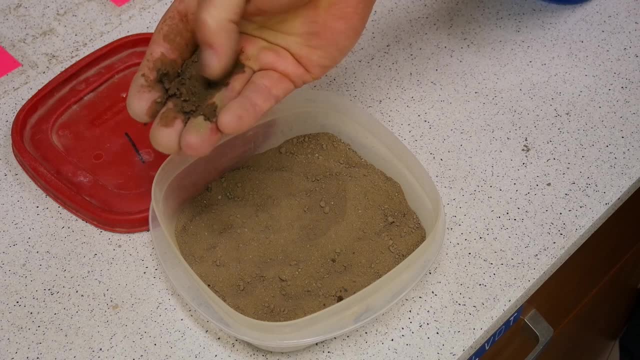 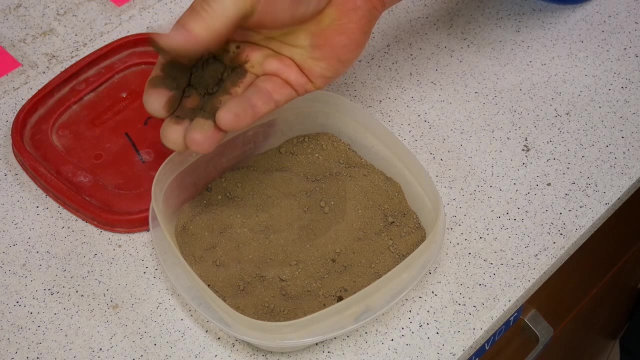 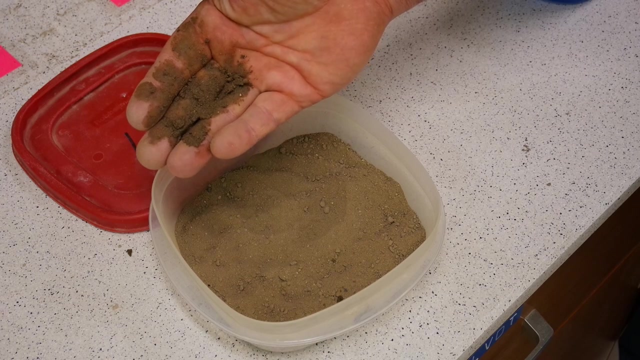 whether it is a 0 to 5, 5 to 12 or 12 and above, as far as the fine goes to determine what your classification is, I will let you look at that based on what you see going on. This is what is going on in my hand. 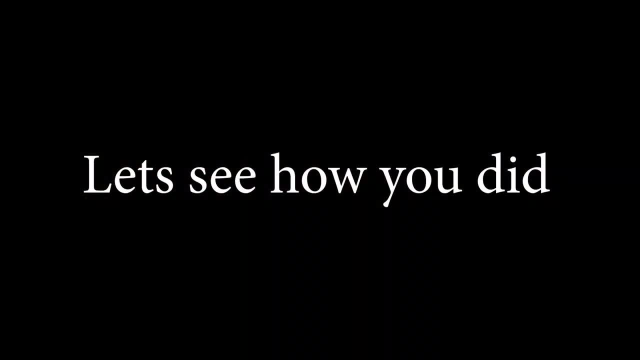 And that is it for sample number 12.. Okay, now that you have had a chance to guess what the materials are, I am going to go ahead and describe again how I would have looked at it and give you the classification for all 12 of these samples. 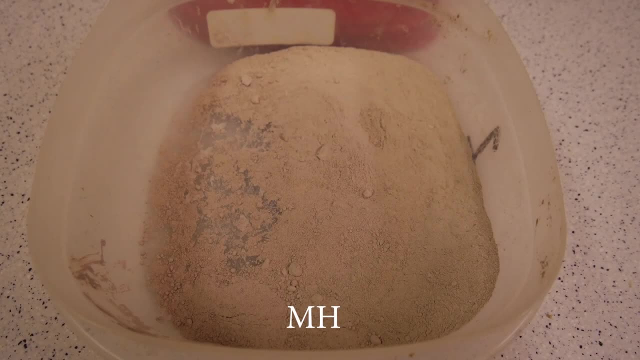 Let's see how well you did So. sample number 1: I basically told you that it is either a clay or a silt, Just because of the makeup and the fines and feeling it, And so, as I feel it, and I describe it as being silky, 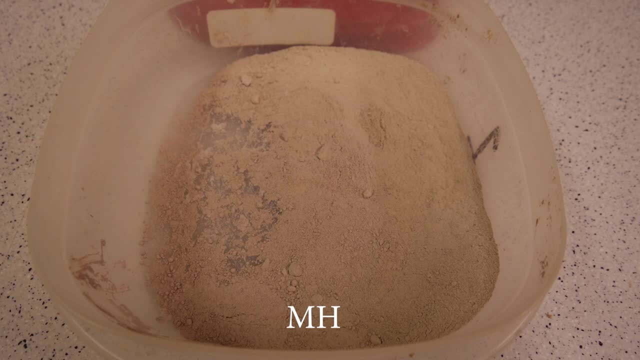 that would tend to make it a silt as far as how I would feel it in the field and what I would determine it to be, And so what I really need to know now is how plastic it is, And so a lot of these samples are going to be moist. 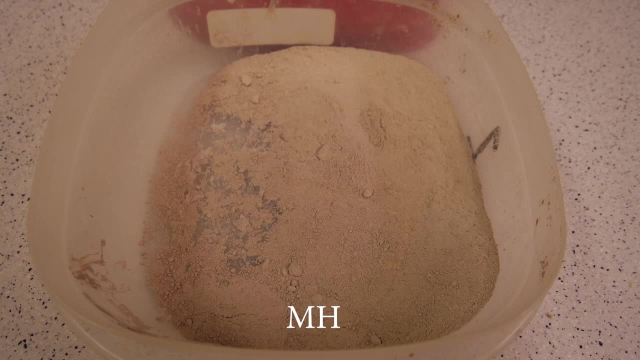 and get them out of the ground, and so you are going to plate them and roll them and see what it takes to roll it down until it breaks. And if it takes quite a bit to do that, then you assume that it is highly plastic or higher plastic. 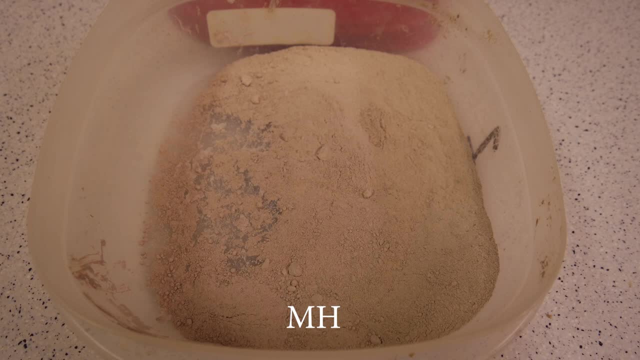 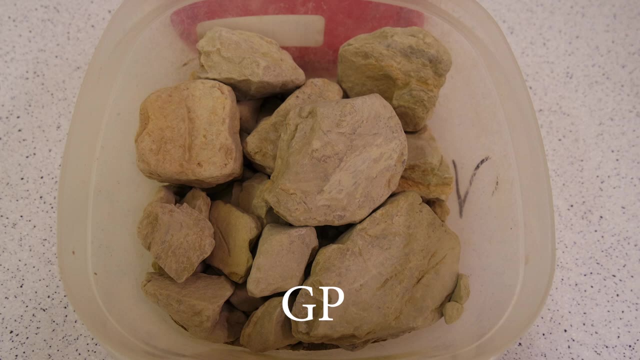 And so in this case this is considered an MH or a highly plastic silt. So as you look at sample number 2, you can tell it is a gravel, right? I mean, it is just the appearance. you know that it is, And so we know that that is the case. 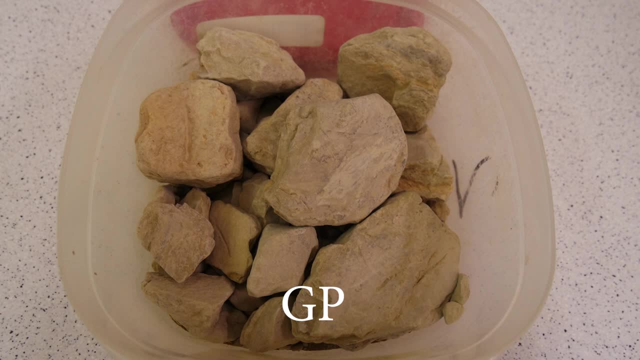 The only question there is is whether it is a well graded or poorly graded material. When I say well graded or poorly graded, whether it is well distributed or whether it is gap graded, And if you look at that, I would tend to think that that material is definitely gap graded. 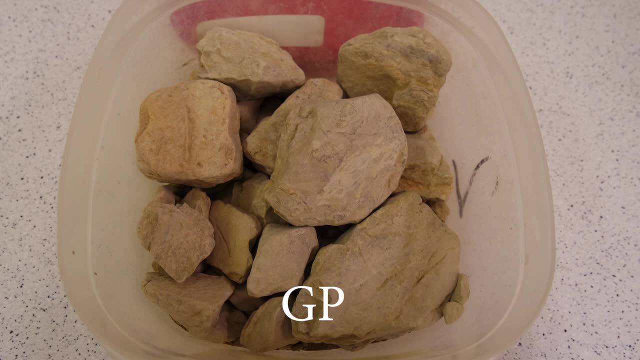 because there is really nothing to bind or fill into it. There is not a distribution of grain sizes. I was making a note of the softness of the rocks because I can indent it with my fingernail and scrape a little bit off, And so it is a really soft rock. 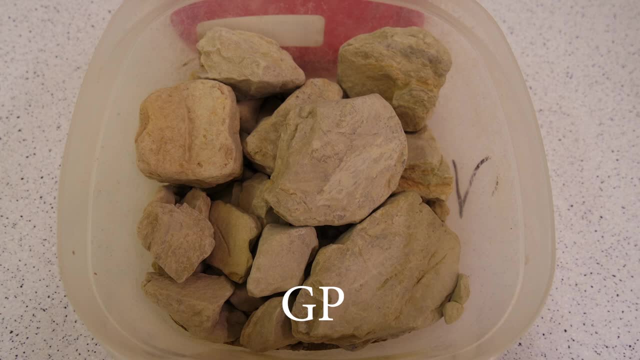 so there even could be potentially a silt stone, because it is really not a sand stone, but there could be a little silt stone to it. But the classification for this should have been GP, which is a poorly graded gravel. Okay, that is sample number 2.. 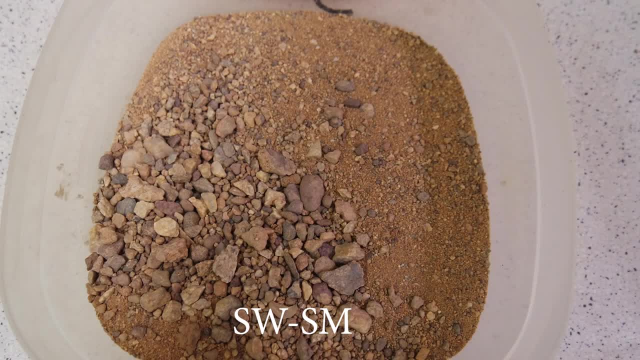 Okay, sample number 3.. It is definitely a sand sample- I mentioned that to you- Whether it is well graded or poorly graded. In this case it is a well graded sand, Even though in the field you typically don't see well graded materials very often. 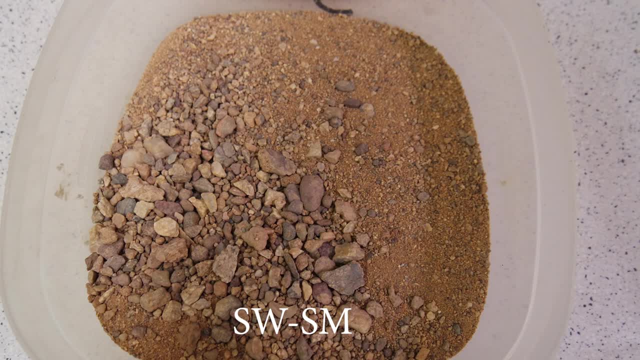 They are usually poorly graded. Usually engineered fills are what you will see as well graded, But this material, because it is not gap graded, is considered a well graded material. And then we got to decide. well, let me back up a little bit. So typically when I see a sand sample, 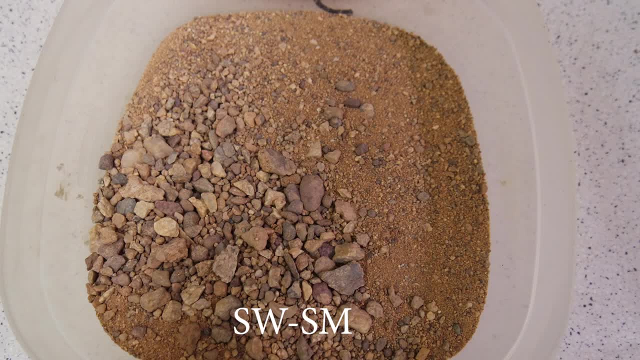 and I see fines in it. I always assume that it would be silts, because silts are coarser than clays, so it tends to follow, And so I would consider the material that was in that that are finer than the 200 sieve as being silt. 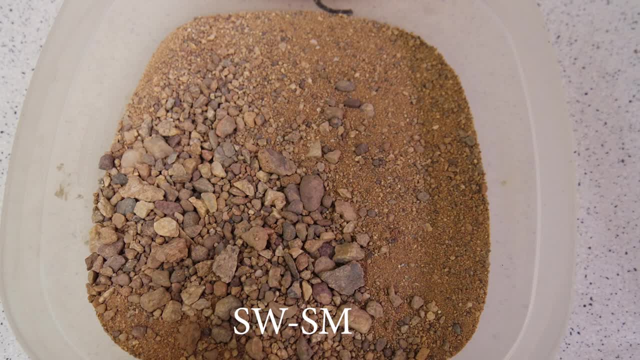 And so we need to determine what our percent of silts are in this material, Because it wouldn't make mud when you added water to it. it would tend to be less than 12%, And so are we 0 to 5 or 5 to 12?. 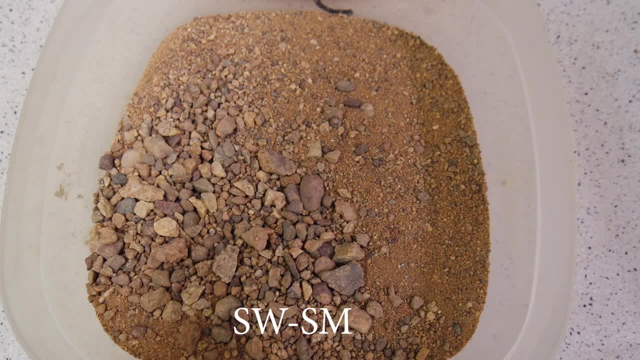 So it does have some fines in it, as I described, And it does, and they are evident, And so I would tend to say it was 5 to 12% if I were to look at that in the field. And so in this case it is. 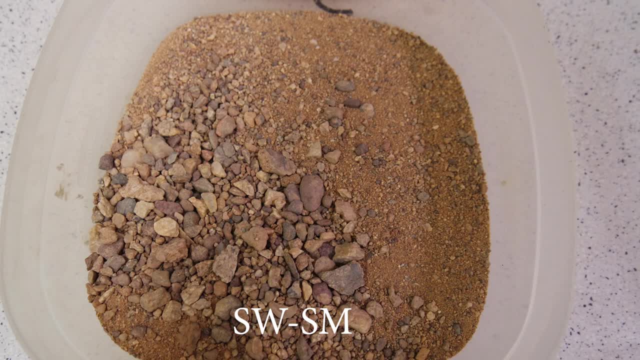 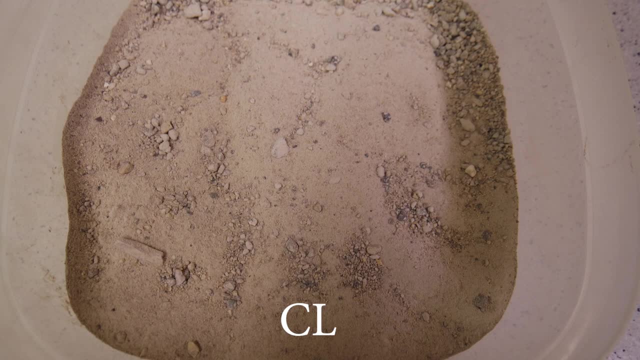 And so the classification on this material would be an SWSM. Okay, so sample number 4.. As I described, the only thing I didn't do in that previous video was roll out a little worm and give you an idea of how much water. 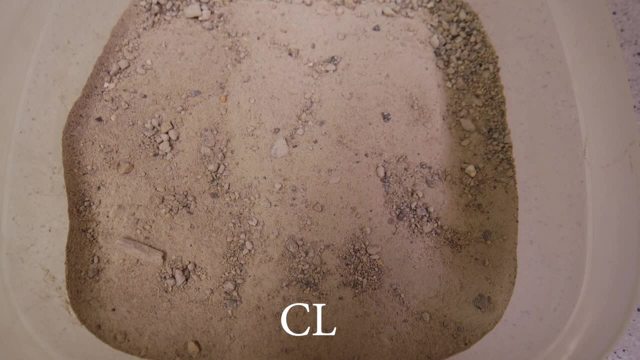 it took to wet it up or get it to its plastic state? Um, as I mentioned, when I looked at it, you look at that water and look how wet that is, Um, and so it didn't take a whole lot of water to wet it up. 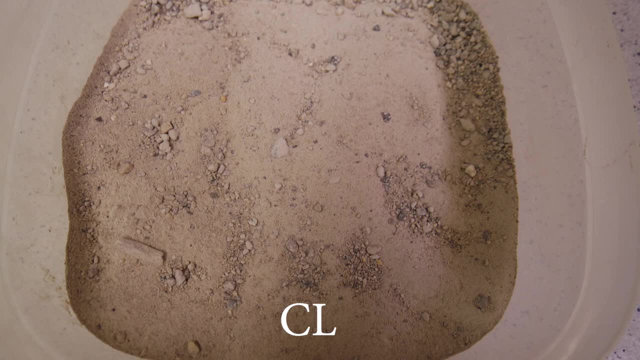 And also you look at it and say: you know, that's pretty, that's pretty sticky. so you're feeling that it's a clay material, Because a clay's materials typically are more sticky than silky. And so we got a clay and even though it has sand in it, 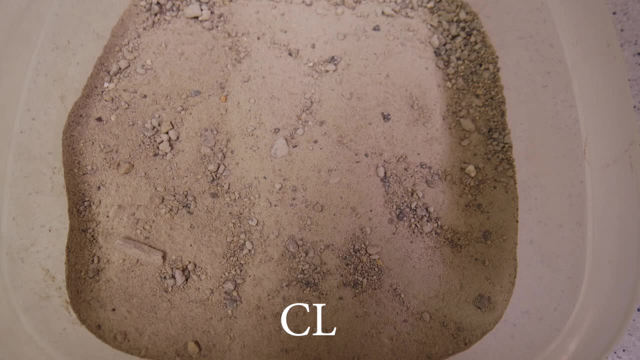 it doesn't have enough sand in it, and you can look at that for the appearance of the dry material to classify it as a sand sample, Because you know there's more than 50% clays And so this would be classified as a CL. 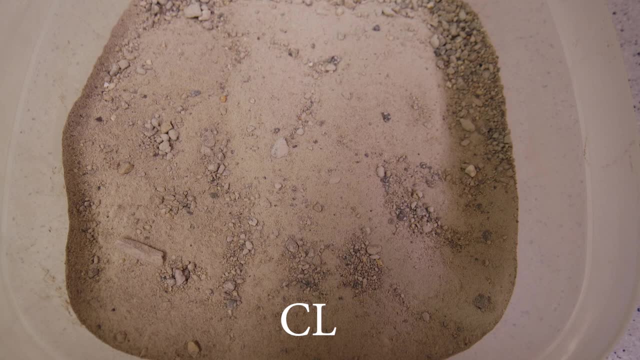 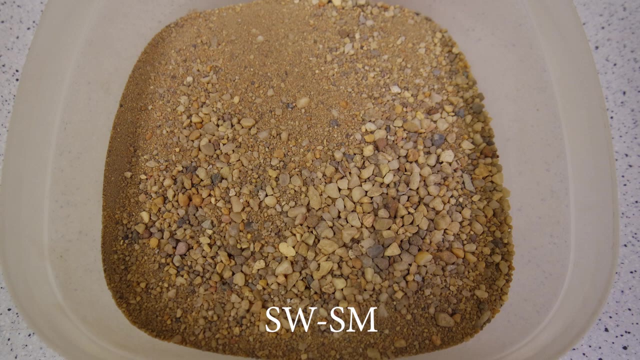 because it's not highly plastic, And so sample number five. it is exactly the same material as sample number three, which is an SWSM, And so we know in this one we have between five and twelve percent fines in it. Um, it looks slightly different. 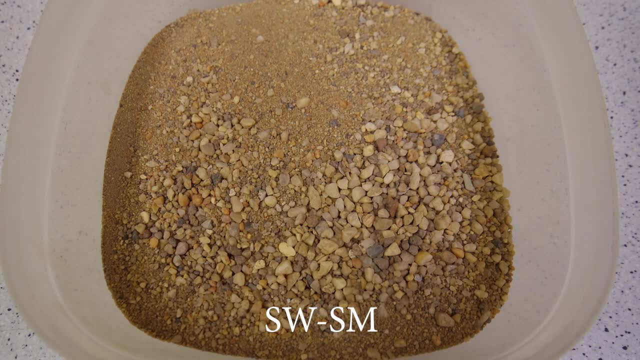 but it is also well graded, And so there's that band you have to work in, that it can be considered well graded or poorly graded, whether it's, uh, well distributed or not, And so it's just a matter of looking at that and identifying them. 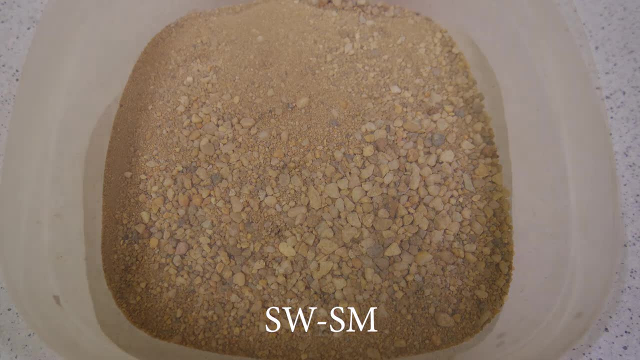 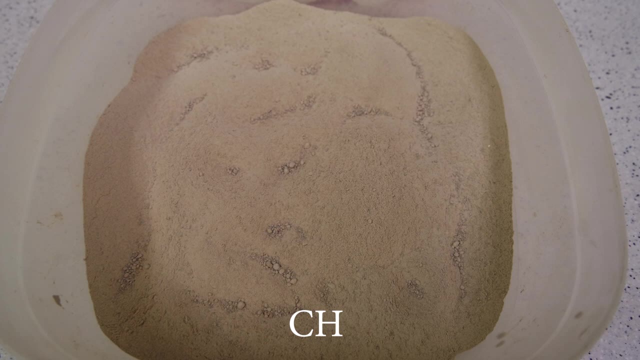 But they're basically the same item. As for sample number six, as we previously discussed, this is more of a sticky material than a silky material, So that would immediately lead me to believe it's a clay as opposed to a silt, And so I added water to it. 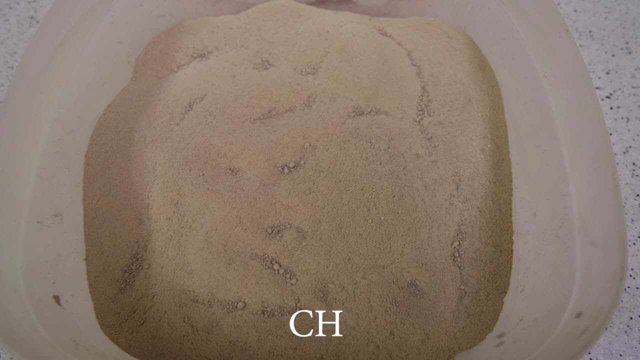 to get an idea of how much water it would take to get it to its plastic limit, And in this case it took quite a bit of water to get there And I could roll it out multiple times, uh, to get it down, before it broke up on me. 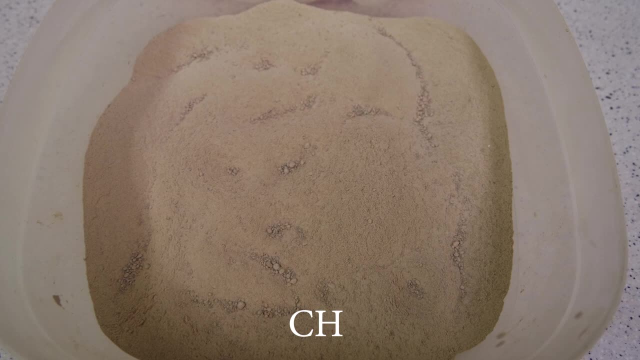 And so we know that it's will take a lot of high, a lot of water, to make it um to its plastic limit, Which would make that really a fat clay, which is called a highly plastic clay or an M or a CH, And so that's what this sample is. 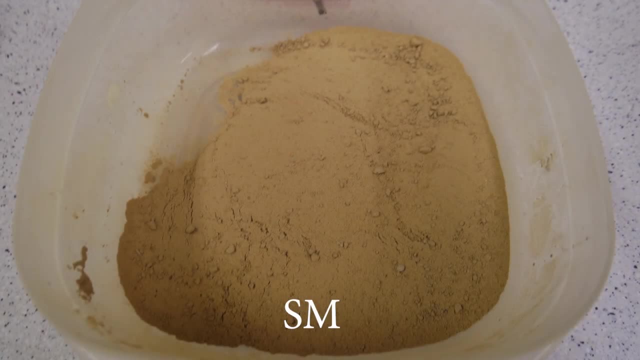 It's a CH. Okay, sample number seven. As we look at that, I noted that there was a lot of sand and a lot of fines in it, And we had to make a determination on whether it was a sand or, in this case, it is a silt. 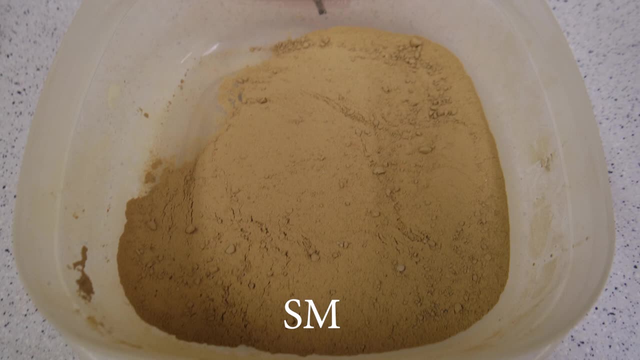 And I already gave you that clue in the uh description video- And so, that being the case, we threw some water on it and tried to roll a worm and saw that it was non-plastic. Just because it's non-plastic does not mean. 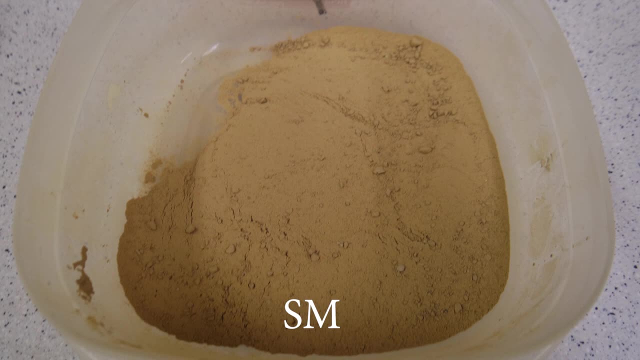 it would be considered more of a silt or more of a sand than more of a silt, But it does show you that it's that it wouldn't be a silt, because if it was plastic, it would be a silt, And so, that being the case, 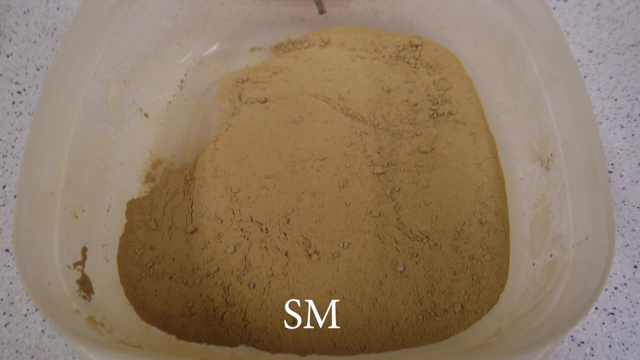 we've got to look at our makeup and decide whether there's more than 50% fines or less than 50% fines. In this case, this sample has less than 50% fines, and so it would make it a sand, But it has more than 12% fines. 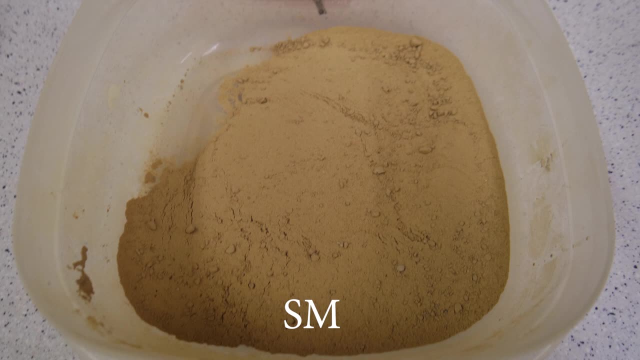 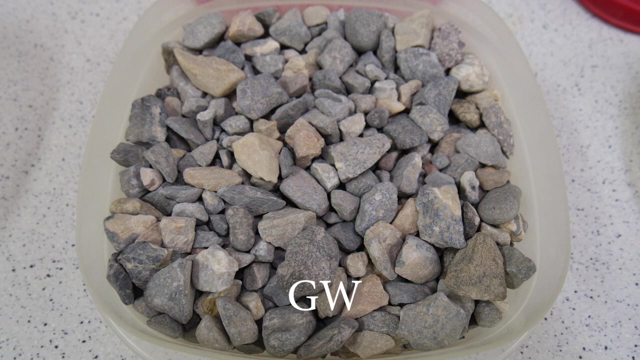 and so it would make it an SM would be the classification. So, looking at sample number eight, I think we're all pretty clear on that. it's a gravel, And so, even though I showed you those fines, those fines don't equate to enough to make it drop into the sand category. 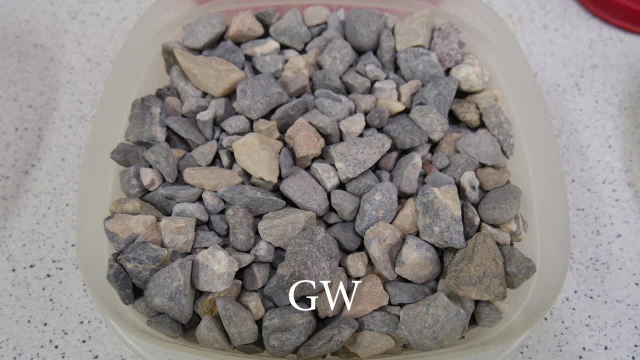 And so whether it's poorly graded or well graded- again one of those hard things to tell in the field. typically, you would never, you hardly ever, see a well graded material in the field. I mean, you do, but it's by and large a poorly graded material. 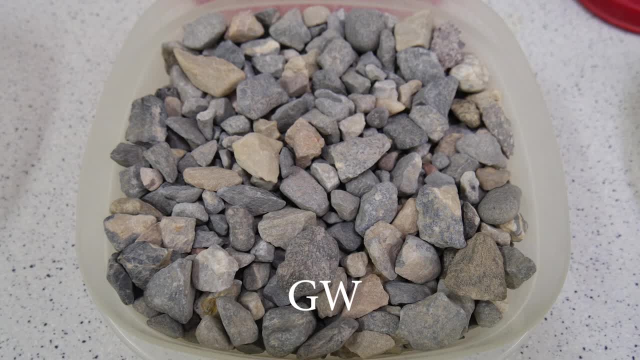 And so if I was in the field, I would typically call it a poorly graded gravel. But in this case- and that's why I showed you the fines- is that if you look at it, you can see that there's a lot of all the different grain sizes. 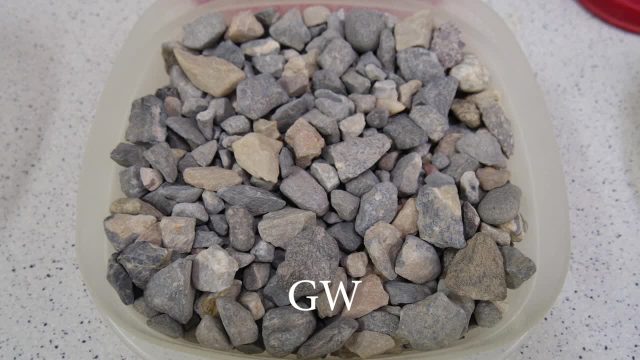 and they'll be able to fill the gaps. so it's not gap graded And so it would. this sample is a well graded material And we know, looking at it, that we have less than 5% fines, And so this would end up being classified. 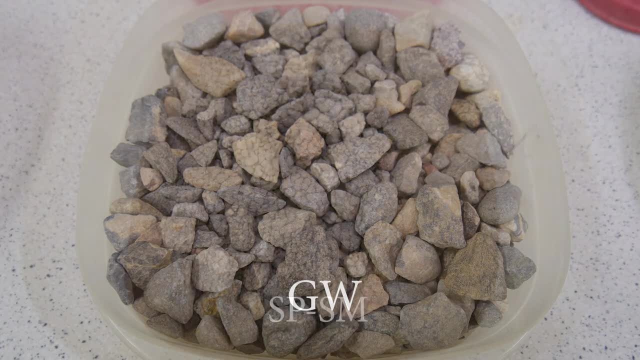 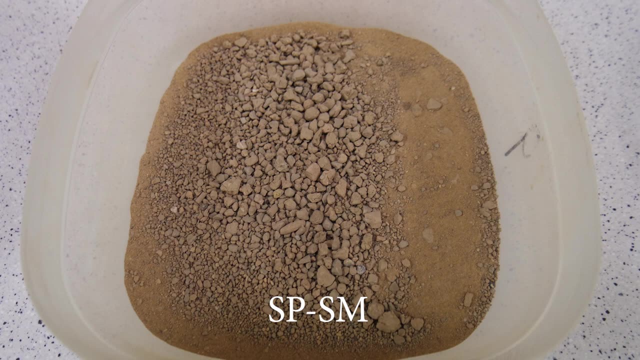 as a GW. So, as we look at sample number nine, I basically let you know that it was a sand sample And that, looking at it, you could tell that it's gap graded, and so you know that it's poorly graded, And so those two items are pretty obvious. 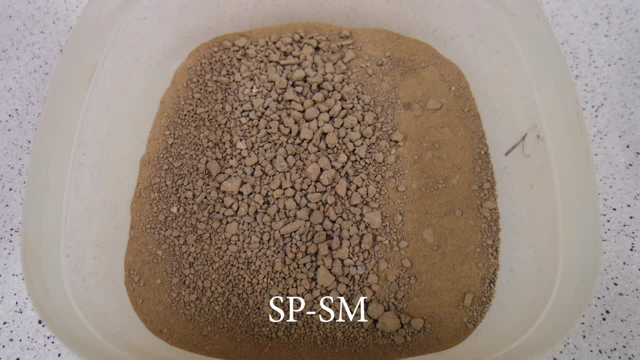 So you know that it's an SP, So a poorly graded sand. The question is, how many fines are in that? And so you look at that: it looks dirty. It doesn't look excessively dirty, but it looks dirty And so it's not clean. 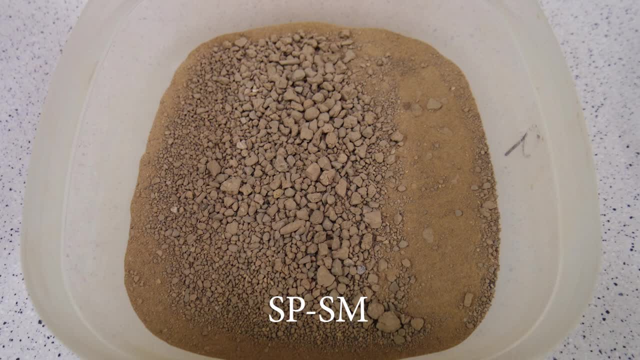 so I would not do zero to five And it's not to the point that it makes mud And so I wouldn't go over 12%. So it's someplace in between. So it's the five to 12% area. So the classification on this. 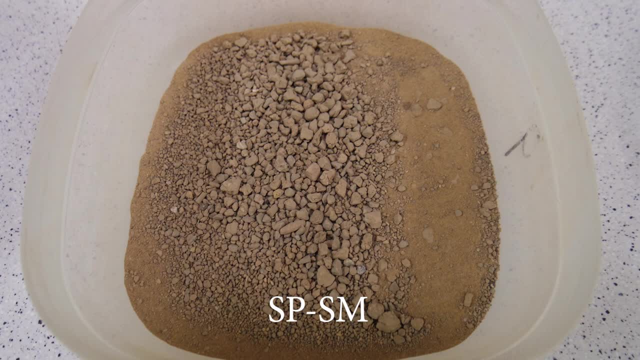 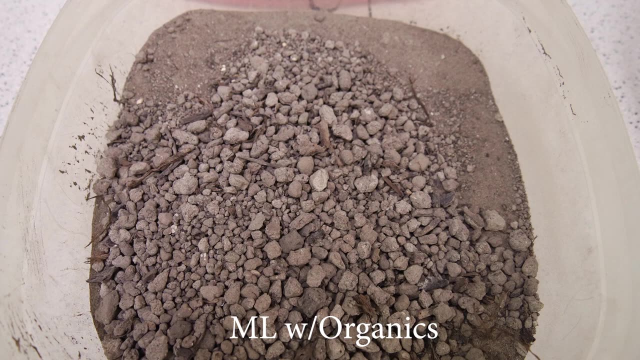 would be an SPSM. So sample number 10 is an unusual sample. You do run across it in the field, where you have samples that have organics, Especially one samples that are closer to the surface, And so the first thing you will do, 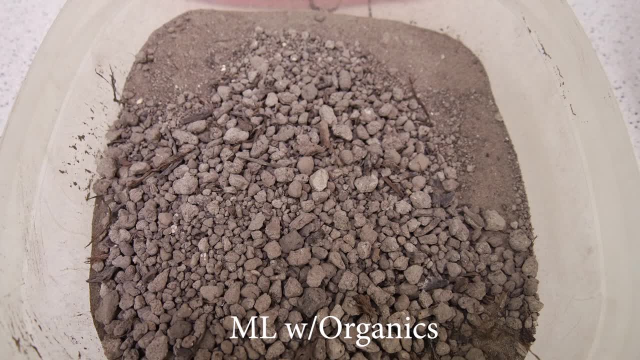 is when it comes out, is you can smell it. If you suspect that there's organics in it, just smell it And you'll be able to tell that organic smell, And so you know there's organics in there. And so the next thing you can do, 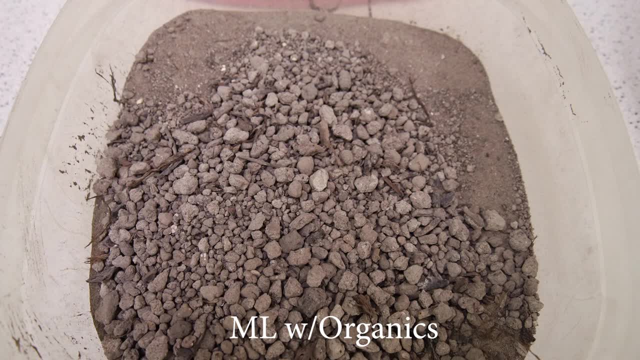 is you're going to look at it as I did. I put water on it. You can watch the water beat up, Which also indicates that there was organics in that sample, And then we added water. As we added the water, we also mixed it up. 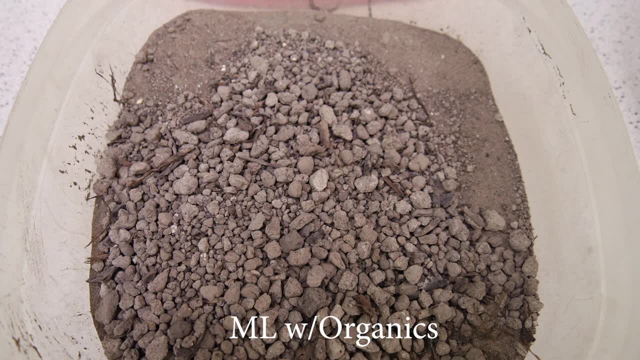 and saw that it was either a silt or a clay. And so, without doing organic loss by ignition, which is basically, you take and you put white gas over a sample, You weigh it first And you burn it multiple times until you have burned all the organics off. 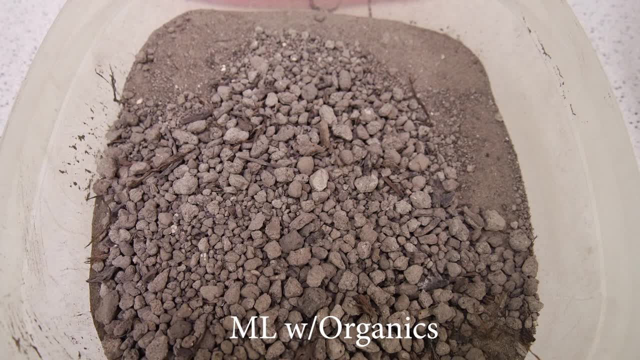 And then you re-weigh it again and see what the percentage of that was in organics. I would be hard pressed in the field to be able to say whether it would be an organic sample or a clay or silt sample with organics. 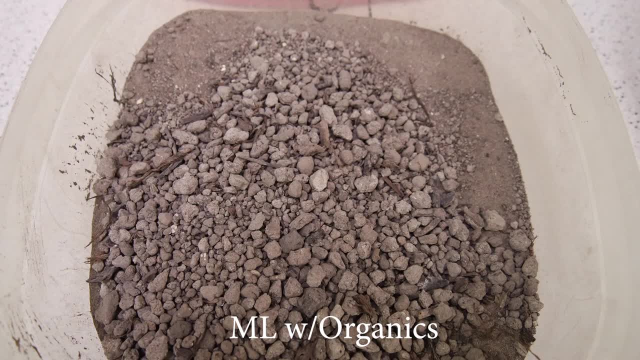 And so, but in this case there wasn't a lot of organics in there, So I would have called this because- and I didn't mention it to you in the video- that that sample was more silky than it was sticky, And so I would have called this an ML. 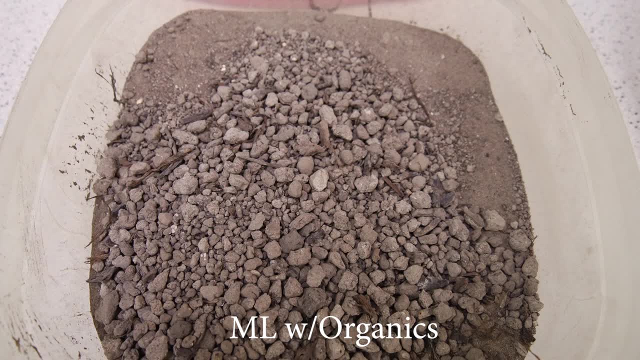 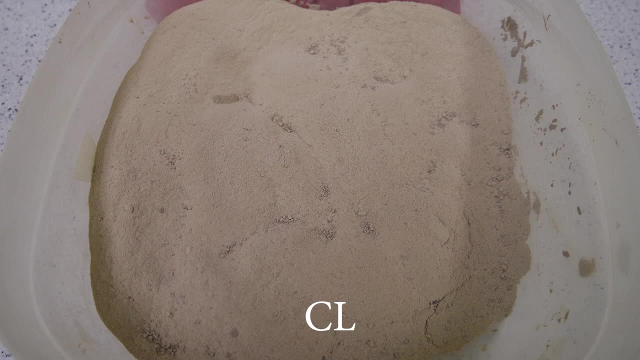 or I would call this an ML with organics. So sample number 11 is pretty straightforward. As I mentioned, it was a sticky material And so as you play with it, you pretty much understand that it's a clay, just from the way that it feels. 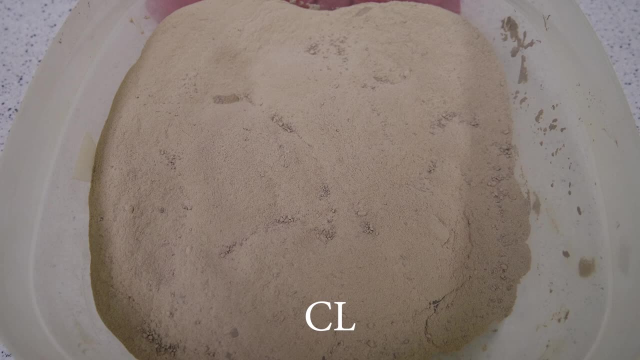 And as you put water into it, you can see how much water it absorbs and how sticky it is and whether or not it absorbs a lot of water, Because a lot of times you're doing this in the field, you're doing it with samples that are already moist. 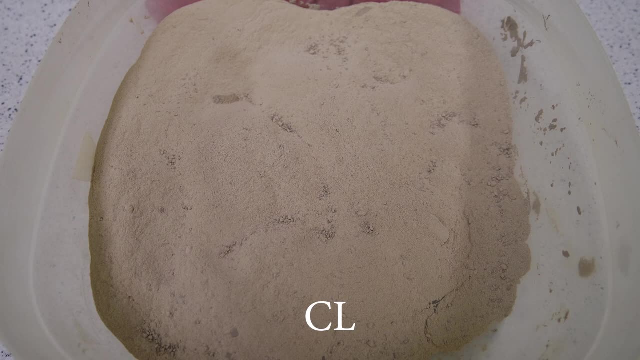 And so you're feeling them and seeing how well they roll out and how long it would take to roll that sample to break it down. This case it wouldn't take a whole lot to roll it down to break it down because it didn't absorb a lot of water.